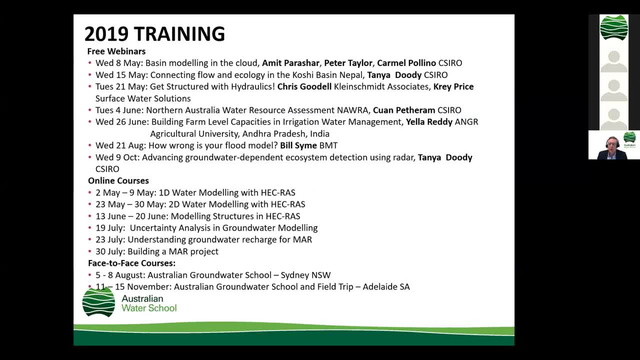 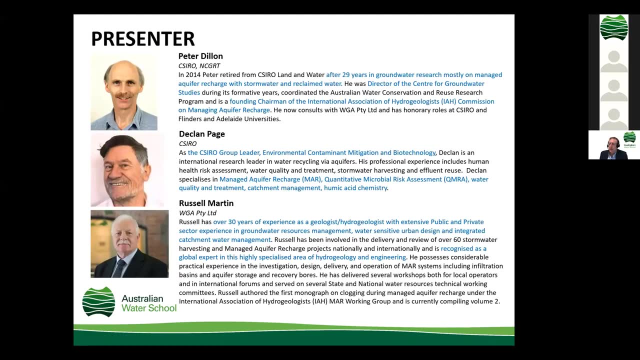 Go on to the IceWarm website, Australian Water School website, and you'll see all the details about that. I won't go into each one, but we cover a vast array of water management issues, as you can see there. Let's get right into this. Three presenters today are Peter Dillon, Declan Page and Russell Martin. So glad to have your company today. More than your company- your input and expertise over many, many years. 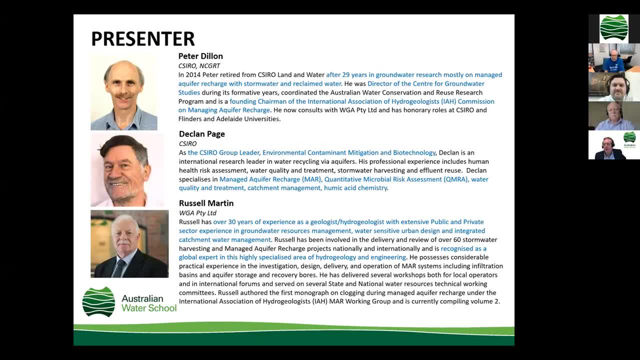 Peter Dillon was from CSIRO and NCGRT National Centre for Groundwater Research. He's been a director of the Centre for Groundwater Research and Training. Peter has 29 years in groundwater research, managing aquifer recharge with stormwater and reclaimed water. director of the Centre for Groundwater Studies. founding chairman of the IAH Commission on Managed Aquifer Recharge. 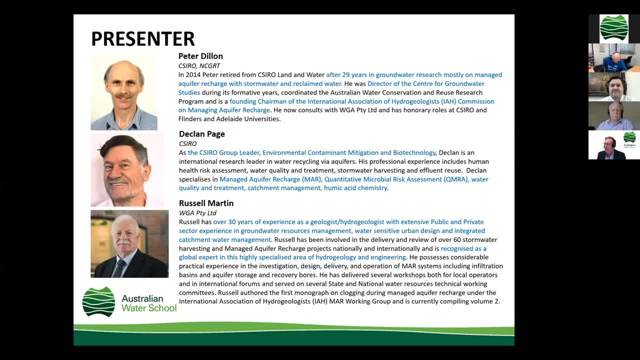 Much more we could say, But thank you, Peter, for joining us. It's a great pleasure to have you. I'll keep going. Declan, CSIRO Scientist Group. Leader at the Environmental Contaminant Mitigation and Biotechnology Group, International Research Leader in Water Recycling. 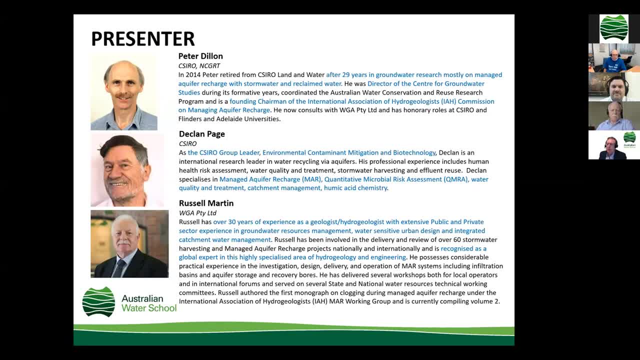 via aquifers. russ martin, from wgap limited, had 30 years experience as a geologist and hydrogeologist with extensive public and private sector experience. there's much more there that could be read, but thank you, gentlemen, great to see you today from um the beautiful sunny adelaide. 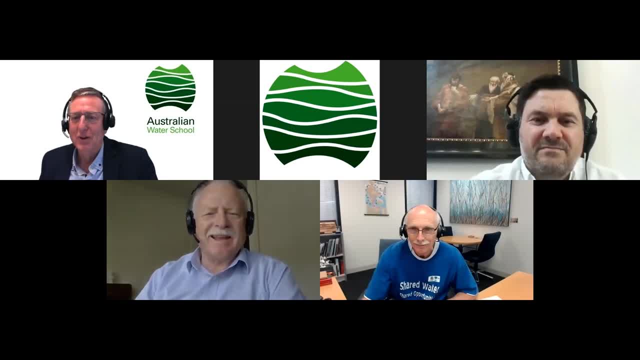 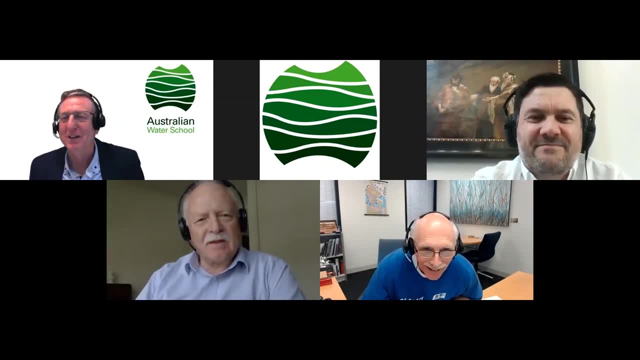 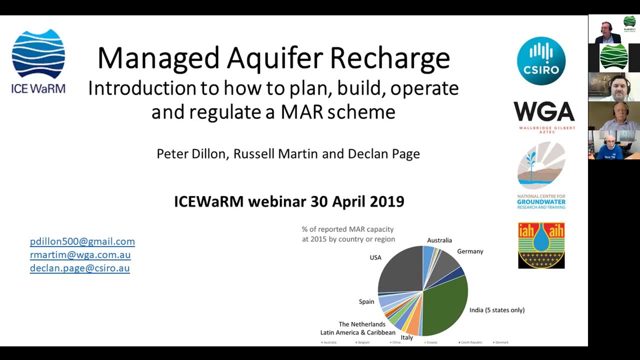 maybe. thanks, trevor. maybe too much sun, not enough rain tomorrow. yeah, we are hoping, declan, i think there's much hope in that statement. i think i think i've had 28 mils all year at my place. let's get right into this. first, off the cap, off the rank is peter he'll. 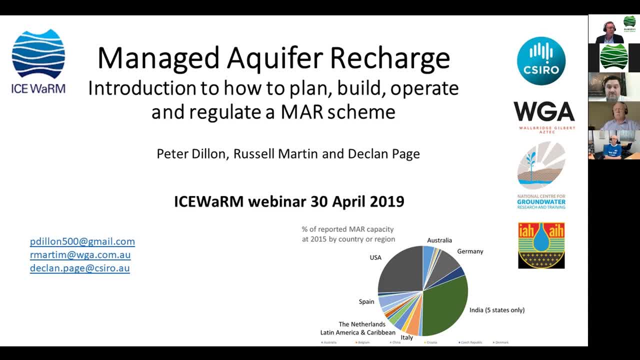 hand over to russ and then declan. uh, as i said before, if your question's coming or discussion coming, we'll interrupt where we uh when we need to. you okay with that, peter, okay with that russ and declan, we'll, um, we'll probably keep the main discussion until, uh, the q a session after the. 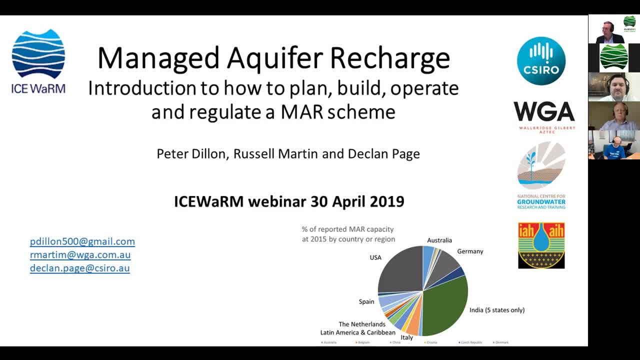 talks. talks are accepted in the 10 minutes each. but that's enough of me. we're going to hand right over to the three presenters, and first up is peter. over to you, peter. thanks trevor. hello everyone. it's so great to see you. uh, ice warm has got technology that you think you're looking at me on a camera and i can see you. 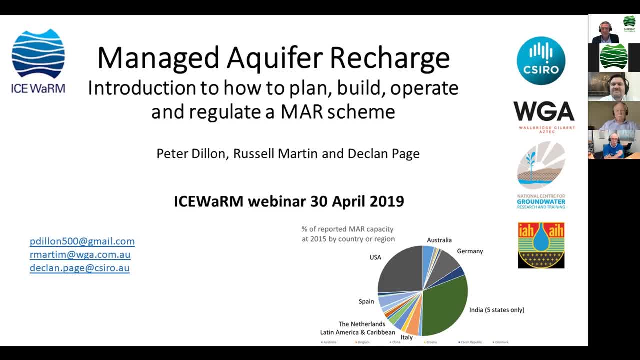 so, um, i'll be watching you. well, we're going to talk today about managed aquifer recharge: how to plan, build and operate and regulate a mar scheme. there's a fair bit of material to cover, so i'll get on onto it, and there are three of us here to 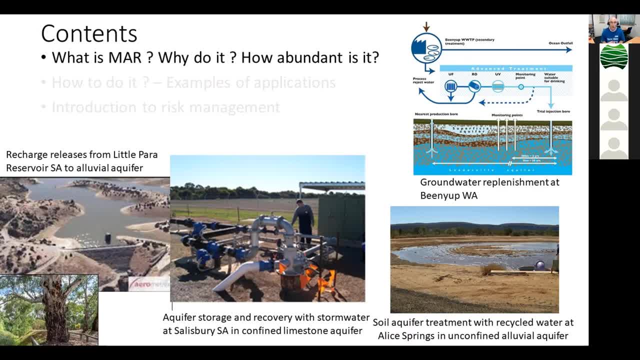 do it, and i'm going to take the first bit about what is ma and why do it, how abundant is it around the world, and then russell will tell us how to do it in 10 minutes, and then declan will lead us in an introduction to risk assessment and risk management, which is very important for us in 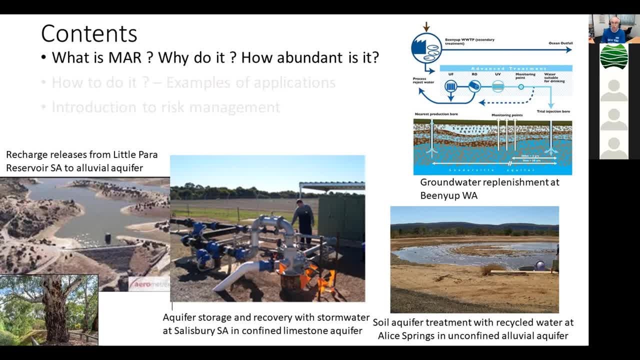 australia and uh, how we've been able to advance managed equity for recharge. so there's some pictures there of different australian projects: reservoir releases on the over here from little para reservoir near adelaide, a stormwater aquifer storage and recovery scheme, infiltration or through soil aquifer treatment with recycled water at alice springs. 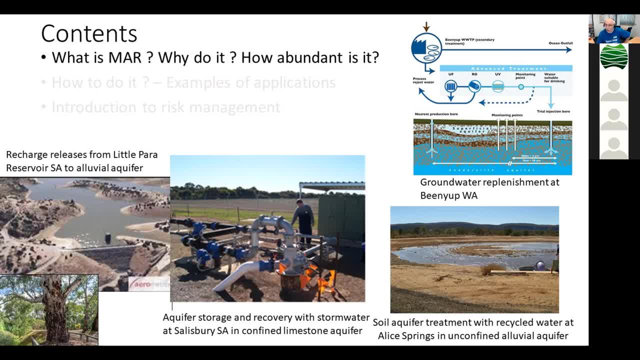 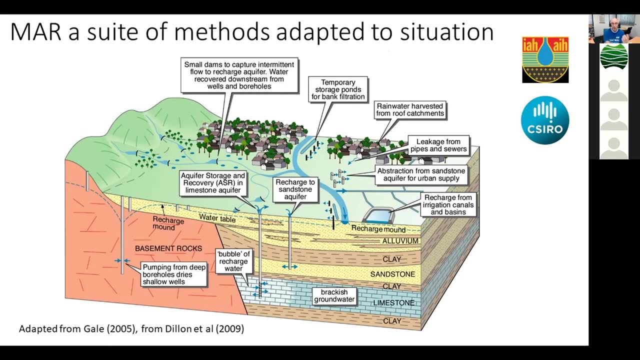 and then this one is. the is a diagram of the benny up groundwater replenishment program in perth, where recycled water is replenishing an aquifer for drinking water supplies. so there's a lot of experience in managed aquifer recharge and and basically it's it's a technique that is for the purposeful recharge of water to aquifers. 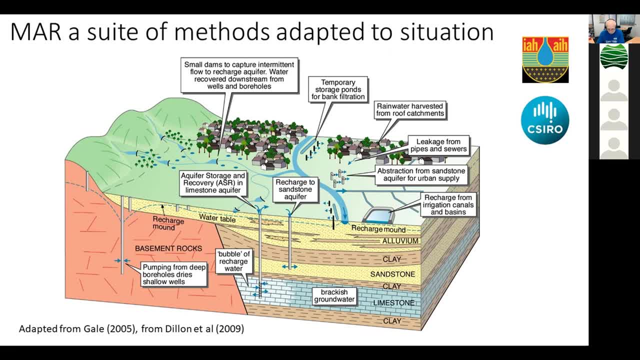 for subsequent recovery or environmental benefit. it's not a method for waste management. it's a way to manage water for the purpose of. this little diagram was drawn up by a colleague, ian gale, from british geological survey some time ago and shows that there are various niches where different types of managed aquifer recharge can. 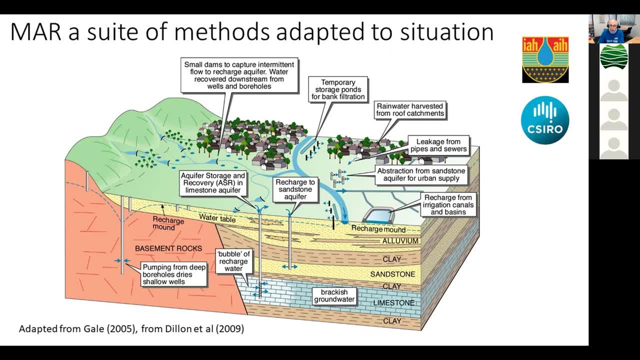 occur. we can see aquifer storage and recovery here in the middle with injection and recovery from one well there are check dams, hard rock areas. i've got a colleague that's just had a paper pub published on the economics and the hydrology of those in the last two days and that's now an 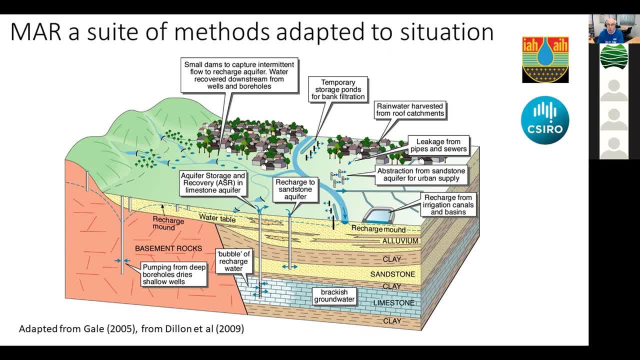 open access paper from the hydrogeology journal durchoura did that in raja stan bank filtration, where people pump adjacent the river to to induce infiltration through the, the alluvium, to get a better quality of water fit for urban water supplies, and there's a whole lot of other methods they're applied. penetration basins and soil Blockchain. here channel galакти П schwauふят is also run by cardiology. on resistance hard such ore classes, high positive plastics, a lot of time expelling bright signs as hydrologic access to high addition脆 nah. 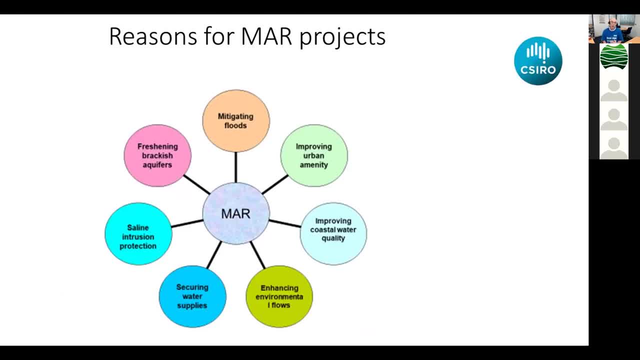 We've got a lot of time where staffs in the area seem to want to take the most time out: aquifer treatment, as I've mentioned. So there's a lot of reasons for doing it: Securing water supplies, particularly increasing security where climate is changing or aquifers are stressed. 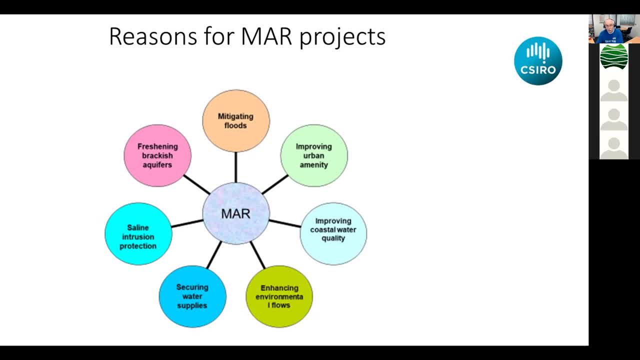 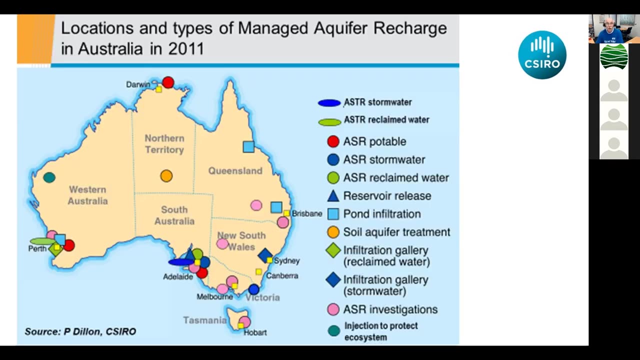 Freshening brackish aquifers to make them useful has been very helpful: The stormwater work in Adelaide which is- there are more than 50 sites now operating generally in brackish aquifers through to enhancing environmental flows, for example. This is an old map but it shows the 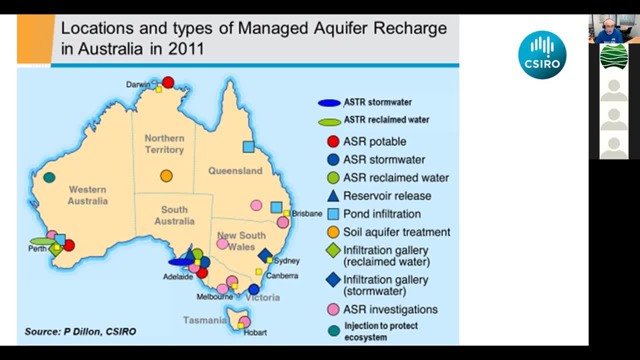 locations in 2011 in Australia where managed aquifer recharge was occurring, of different types, and there are basically two clusters, Perth and Adelaide, and more recently, Melbourne has taken up the cudgel- and they're sites where there's a demand for water, where aquifers have. 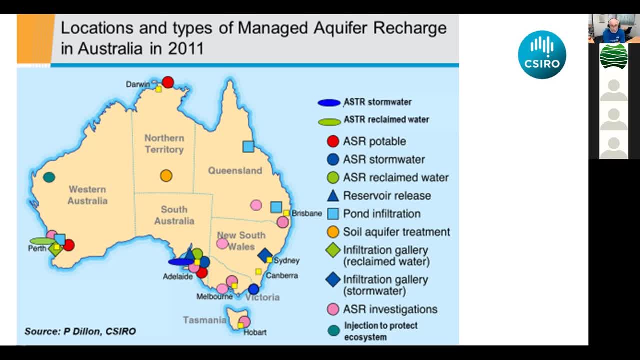 been stressed, where they've been regulators that have been forward thinking, where they've been entrepreneurial councils or water utilities or industries that have taken up the initiative and decided to invest in in these techniques and you can see it's gradually spread around the rest of the country and there 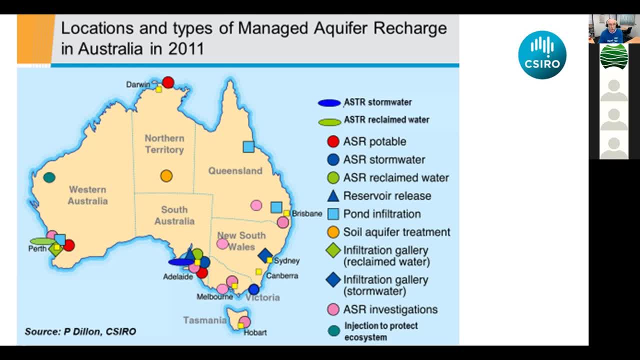 are sites, say, for example, in Western Australia, where you can see that there's a demand for water and there's a demand for aquifers and there's a demand for water, delicate use of water, a outside natural gas that has released, so there's a whole range of types of waters being used to in different ways for managed aquifer recharge. 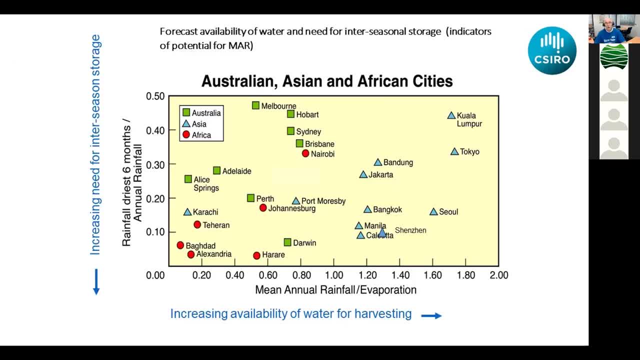 Okay, No other questions tomorrow on this very important topic. Thanks everyone, Thank you. Thank you again. Thank you again to everybody for having us here. Jim goes to the microphone And this is a bit of a snapshot of different cities looking at the meteorological characteristics. 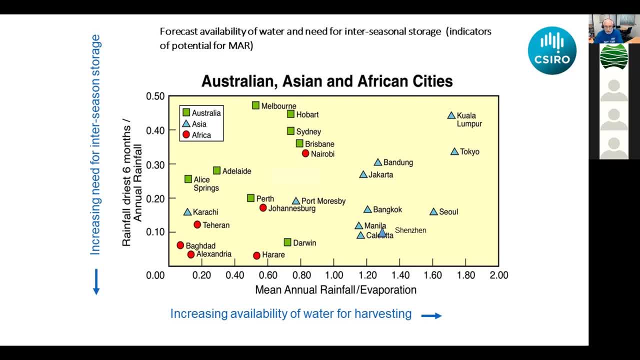 And left to right. on the horizontal axis is increasing wetness mean annual rainfall divided by evaporation, And on the vertical axis is the rainfall in the six driest months continuously divided by the annual rainfall. So the higher you go on that, the more even the rainfall is distributed in a year. 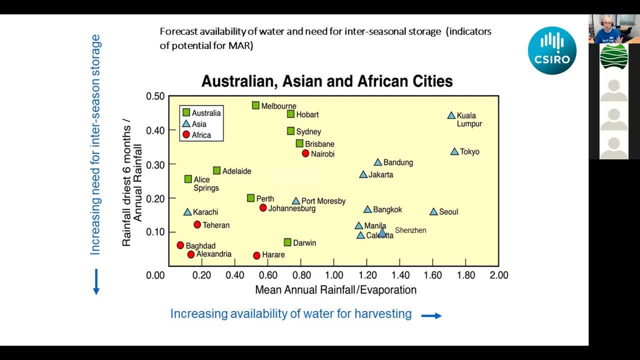 The lower you go, the more un-uniform it is, and so there's an increasing need for storage of water, And what we typically see is that, in the places that are wetter managed, aquifer recharge is typically constrained by aquifer availability. 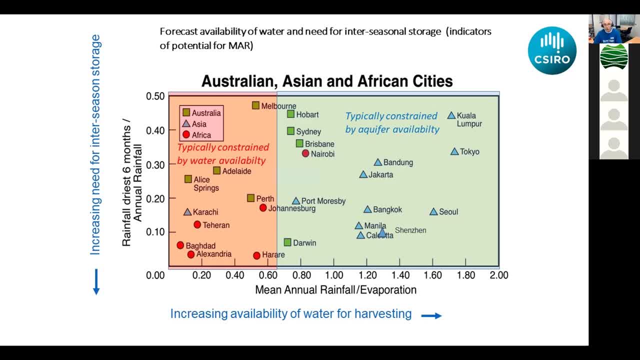 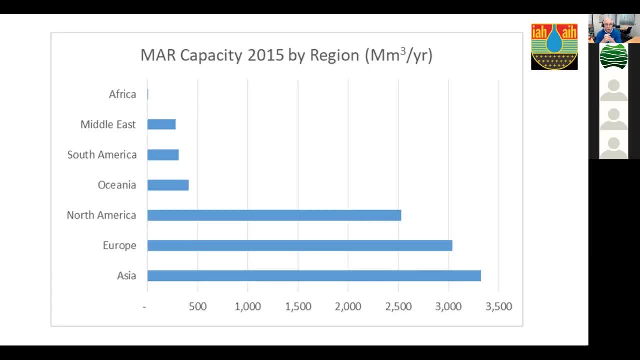 And in the drier areas it's typically constrained by water. A working group of the IAH Commission on Managing Aquifer Recharge got together and did a study of how much managed aquifer recharge was taking place around the world And we looked at it over a 60-year period and as of 2015, by region. we can see that there's quite a spread. 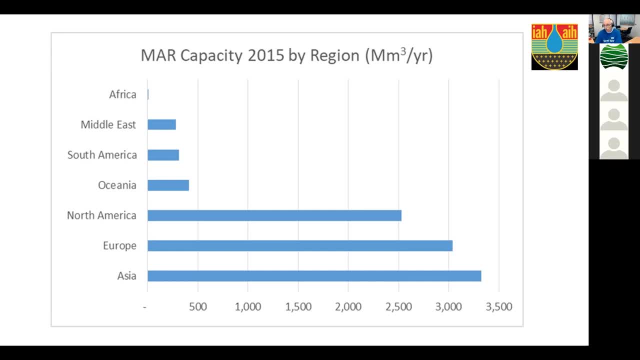 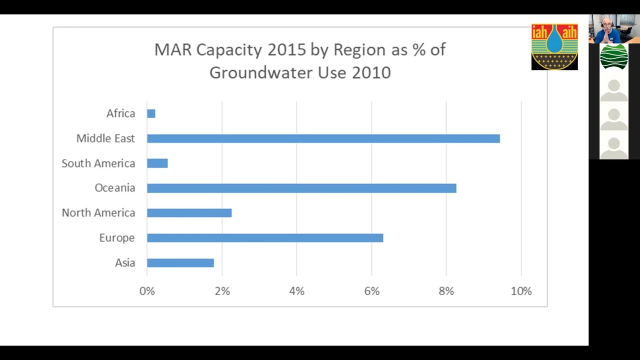 The units here are in million metres square, So this represents three cubic kilometres a year here and it was about 10 cubic kilometres a year in 2015 across the world, with North America, Europe and Asia dominating. When we look at man-hour capacity by region as a percentage of the groundwater use in that region, we see a different pattern emerges. 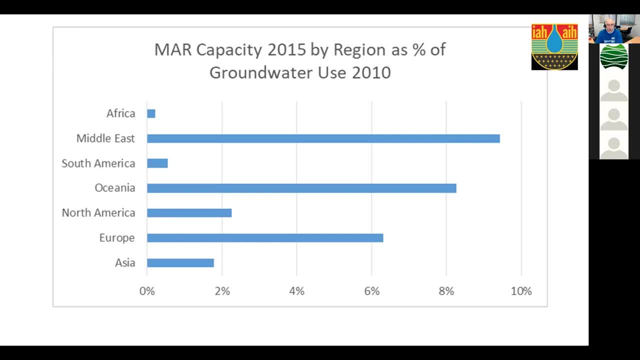 Where the Middle East is the dominant user, with about 9% of its groundwater use, is being replaced by managed aquifer recharge. Oceania, which includes Australia and New Zealand, 8%. Europe, about 6%. There are some countries in Europe that are operating between 25% and 50%, depending on the way that you account for bank filtration. 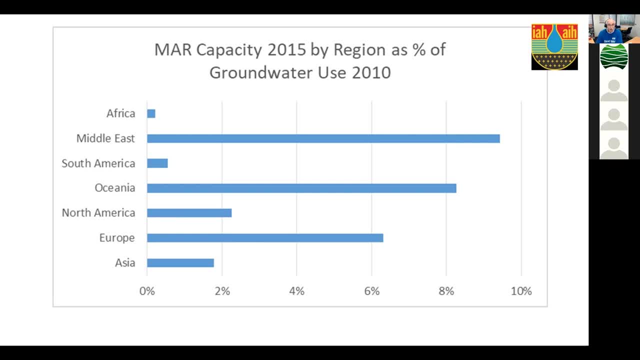 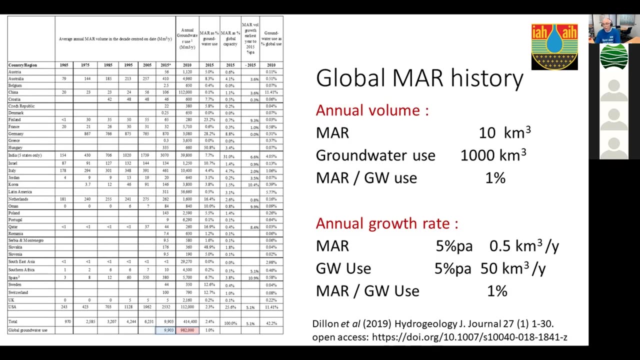 But we see that there are other countries like Africa, South America, North America and Asia in general as a whole where there are huge opportunities for expanding managed aquifer recharge. So the study that was done has been published in the Hydrogeology Journal early this year and it's an open access publication. the reference is there. 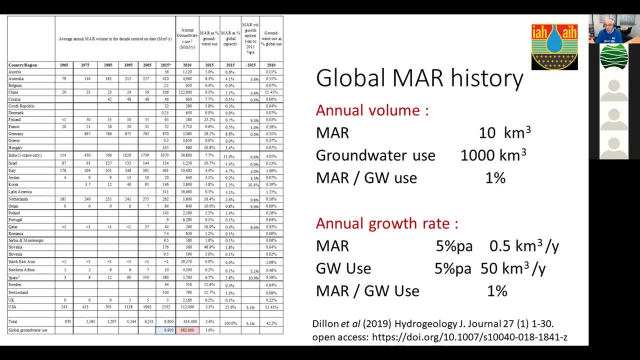 So about 10 cubic kilometres a year of managed aquifer recharge, compared with 982 or 1000.. So about 1% of groundwater use is the current MAR And the growth rate has been over recent years 5% per annum for both managed aquifer recharge and groundwater use. 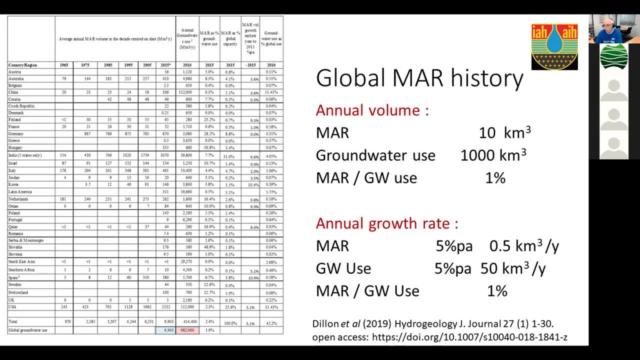 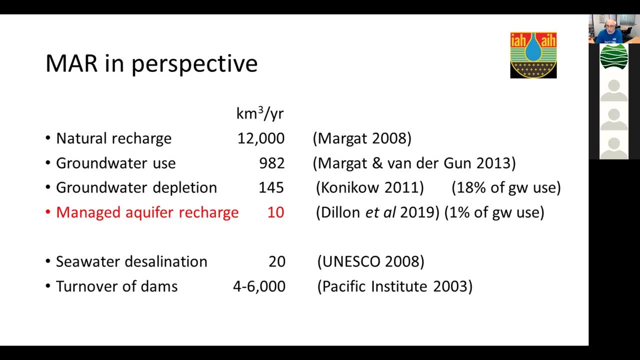 So groundwater use is actually growing globally at 50 cubic kilometres a year, compared with 0.5 cubic kilometres per year. So MAR is by no means keeping up with the increase in groundwater demand, And so we would expect to see groundwater levels will continue to deplete. 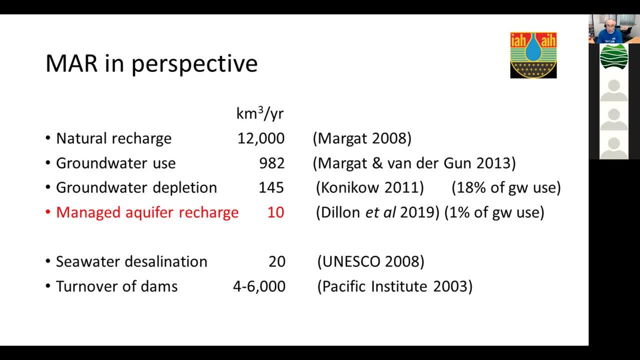 And, as Connor Cow observed, 145 cubic kilometres a year of groundwater depletion caused by the amount of groundwater use. So MAR is not even close to 100 cubic kilometres a year. It's not even close to 100 cubic kilometres a year. It's not even close to 100 cubic kilometres a year. 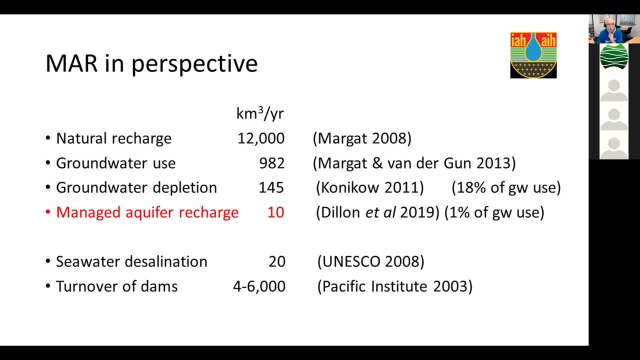 It's only about 8% or less 7% of the groundwater depletion, let alone the groundwater use, And we compare that with seawater desalination and turnover of dams. MAR is pretty small scale at this stage but clearly there's potential for growth. 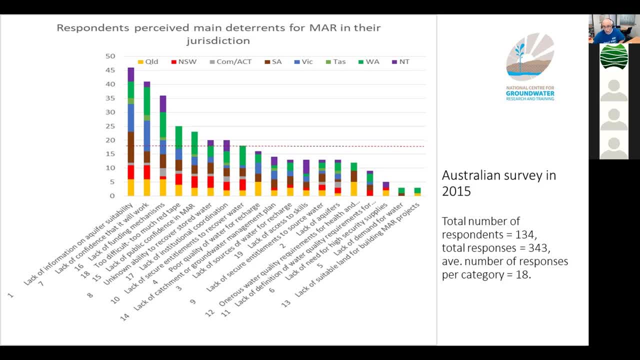 Just a quick snapshot from a survey that was done in Australia in 2015, with 134 respondents from various states, About what was the main deterrent for MAR in their jurisdiction, in their state, And we say that the dominant one was lack of information on aquifer suitability. 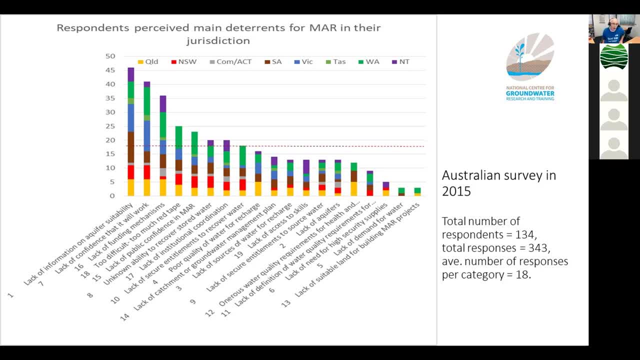 Which is a bit surprising for a first world country. But obviously people believe that they need to know more than they currently do or they haven't really started looking yet. Lack of confidence that it will work. Lack of funding mechanisms: Too difficult. 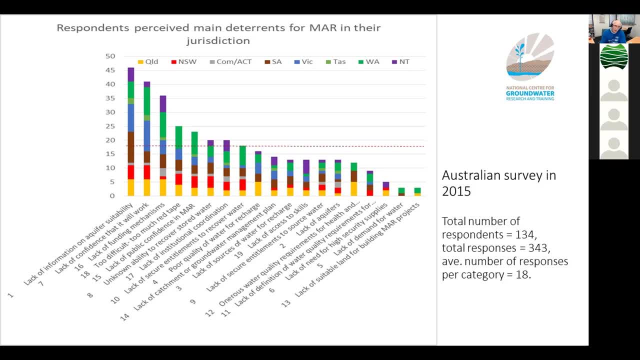 Too difficult, too much red tape. lack of public confidence in MA. unknown ability to recover the stored water. lack of institutional coordination- this is for gaining entitlements to operate, lack of secure entitlements to recover water. So they're the dominant ones. and then there's a whole lot of others that people throw up as reasons. 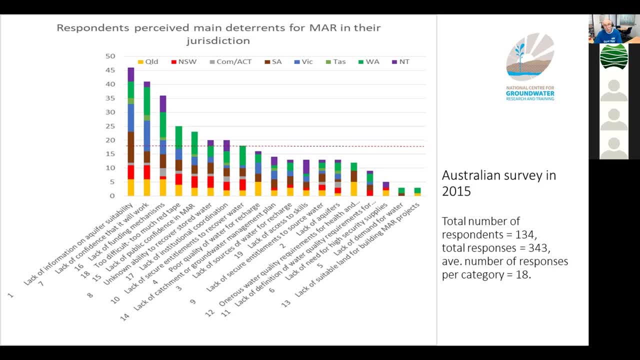 But I guess they're the things that we should probably be working on if we're going to make MA more taken up, not only in Australia, but other countries might have different answers to that, But these are things that we should probably be addressing. 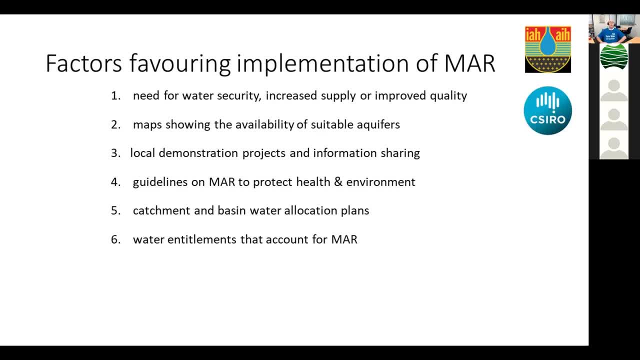 And so the factors favouring the implementation of MA: firstly, the need for water, for water security or increased supply or improved quality, And secondly, maps that show the availability of suitable aquifers, local demonstration projects and information sharing. you saw from that clustering of the maps in Australia there's very broad opportunities for managed aquifer recharge in Australia. yet it tends to happen in clusters because once people see a local demonstration project they get more interested in that. they tend to believe that it's possible. 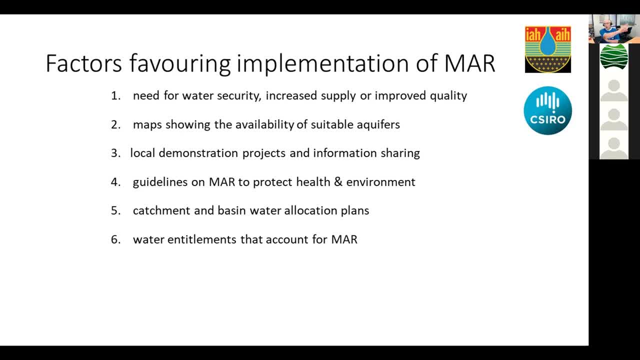 Because if it's happening in some other city, well you know they've got different aquifers over there and perhaps we really can't. you know, it may not be possible for us Guidelines on managed aquifer recharge to protect health and the environment, and Declan will be talking more about the Australian guidelines later, so I won't say any more. 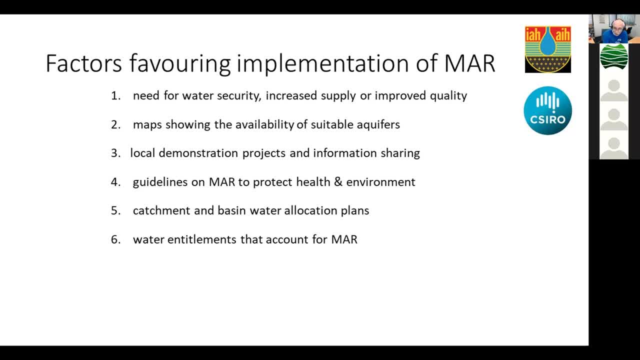 Catchment and water and basin water allocation plans are pretty important for having sustainable managed aquifers, Aquifer recharge operations and in many places they don't exist and there's considerable uncertainty about the availability of water and water entitlements that account for MA. 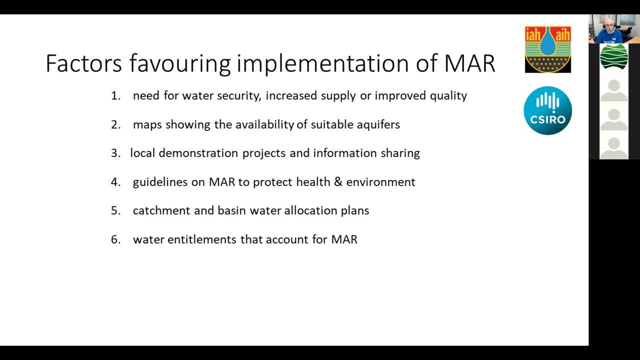 So they're things that, if we were to say, yes, there's a lot of managed aquifer recharge taking place, it's growing at 5%, but it's growing at a much smaller rate than that of groundwater use, What would we need to do? 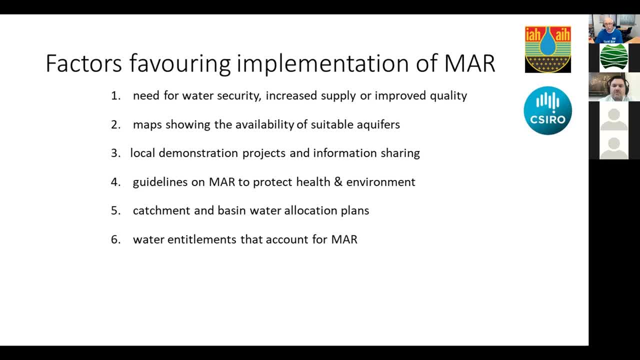 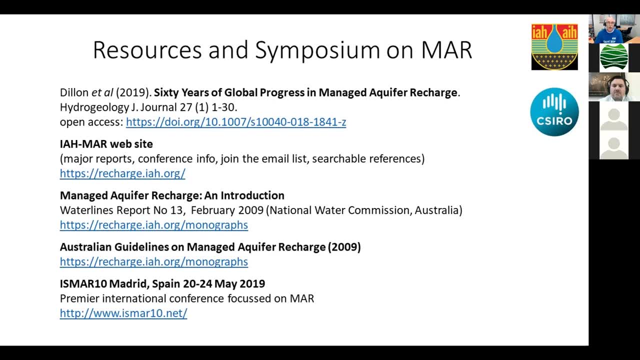 For MA to become part of the equilibrium, part of the sustainability for groundwater in the future. here are some of the things that we could work on. Okay, so here are some resources that are available for you that I've mentioned in this talk. 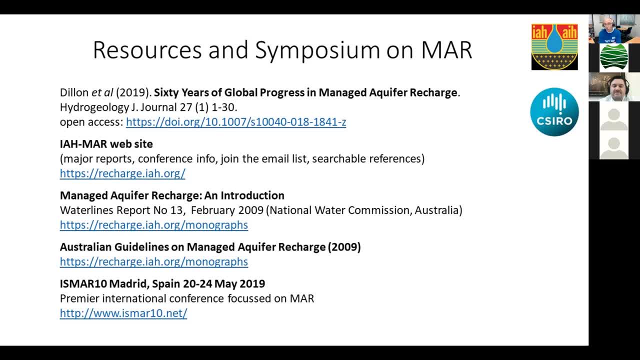 I understand these slides are going to be available to you later, so you don't have to write things down in a hurry, but this is available to you as a resource, courtesy of IceWarm. And that brings me to the end. I hope you've enjoyed my talk. 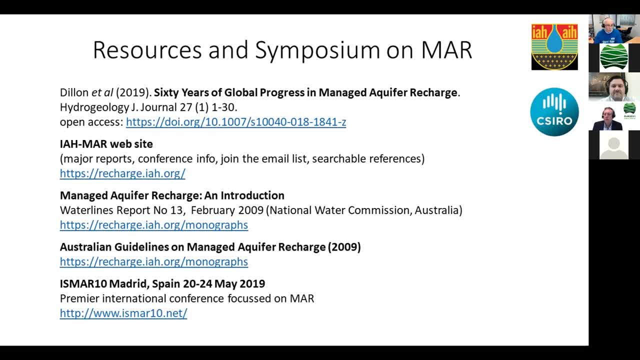 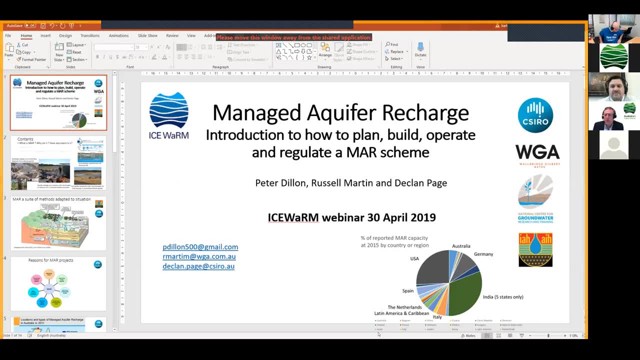 I don't know if there would be any questions before we go on to our next talk. Well, there's one or two just here. Thanks, Peter. That's been a terrific rundown and shows a vast amount of experience coming to bear, as I'm sure you'll all agree. 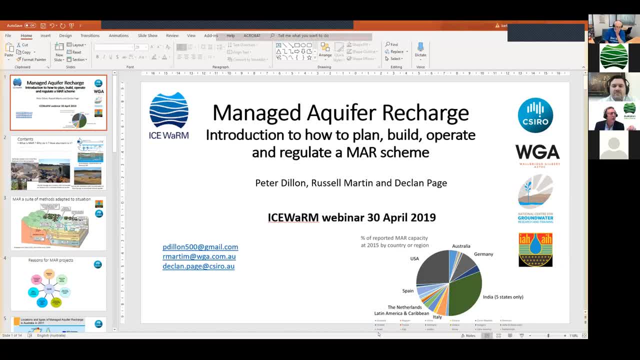 Maybe we can just take one or two of the questions on the board right now. What was the name FORU in New South Wales? what was the name of the paper on the economics? Maybe we could type that in as an answer later, Peter. 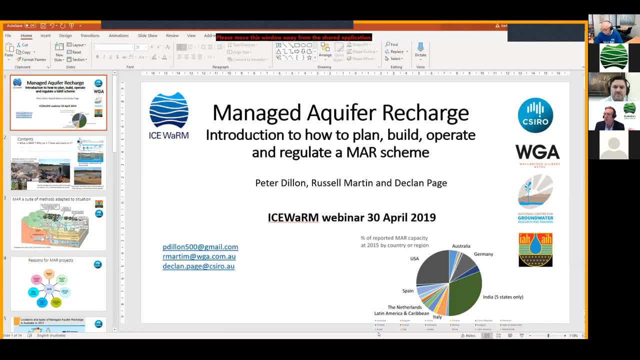 The economics paper. Yes, yes, I'll type that in. That'll be all right. Stand by FORU, that'll come through. One question here on the uses for MAR. One of the economic justifications for MAR in Kabul City is reducing the rate of subsidence. 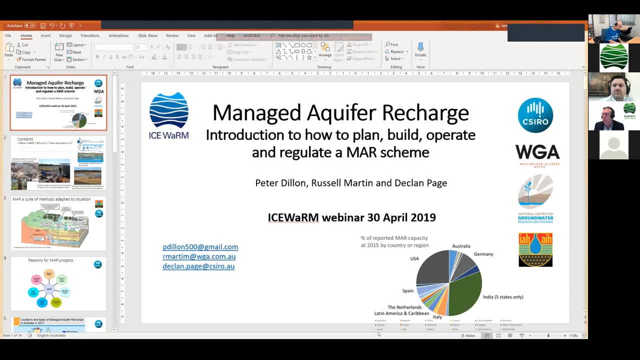 Has this been a driver for MAR elsewhere? Maybe Russ or Declan or Peter might be able to give us some clues on that. What do you think, Declan? I have It hasn't been in my experience, but certainly there are many places in USA, Mexico and others that have got massive amounts of subsidence. 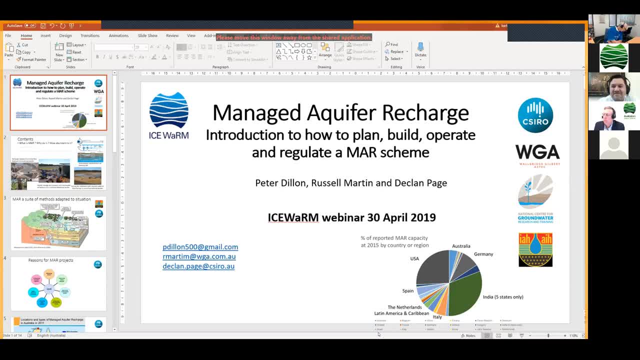 I don't know if you'd necessarily be able to get the volumes in there to have a meaningful impact. Russell, Yeah, you're right, Declan. Both the US and Mexico are key areas where they've been looking at managed aquifer recharge to not restore subsidence but probably prevent any further subsidence. 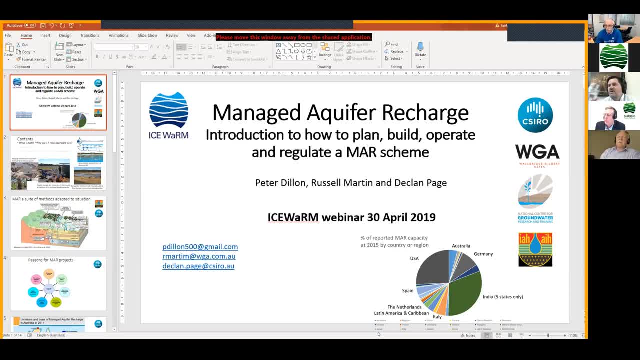 It's in its early days yet, and so the jury in terms of information is still out, but it's certainly being looked at in those localities. Any comment, Peter, on subsidence? Yeah, I've got a comment on it. 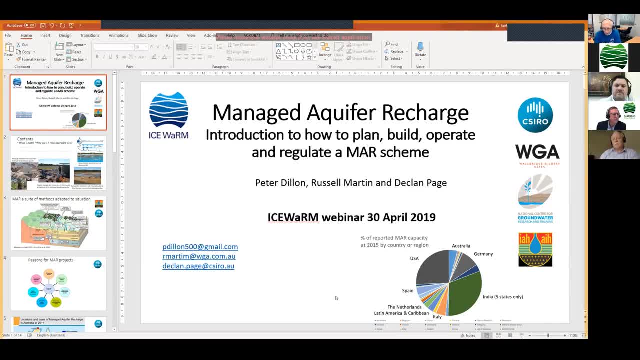 I think it's a foolhardy plan to think that managed aquifer recharge can overcome land subsidence, because the land subsidence is caused by the extraction. If the land subsidence is being caused by extraction, because if you're putting water in and repressurizing the aquifer, basically the people that are pumping water out are spending less on energy- 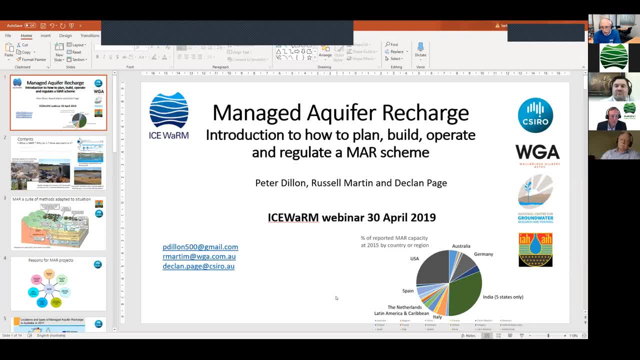 So I would think that demand management is absolutely critical to the control of subsidence and managed aquifer recharge can play a supporting role, and there are various ways. Perhaps we could go through in the course but in which you could implement a MAR program as a consequence of a demand management program being established. 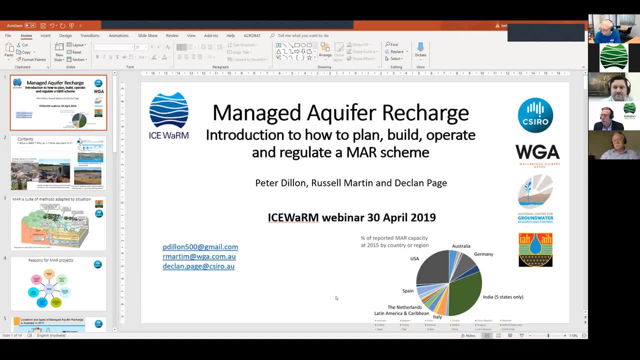 Yeah, look, maybe we'll leave the questions there and we'll keep moving with the talks. now We're going straight into Russell's talk now. So thanks a lot for your questions. everybody, Keep them coming. So look, I see the other questions there from everyone. 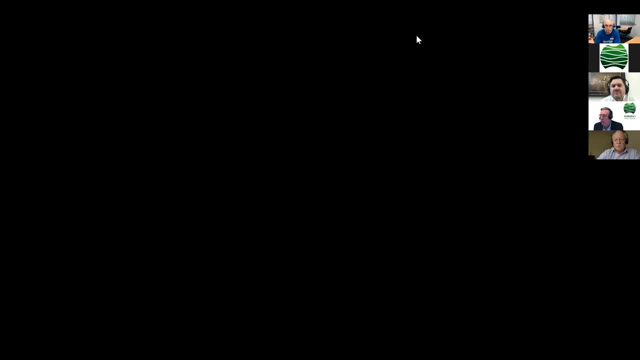 We'll come to them. stand by, we'll get to them, but maybe over to you now, Russ. Thanks Trevor, And Peter has set me a little bit of a task to try and deliver 30 years worth of experience in a minute. 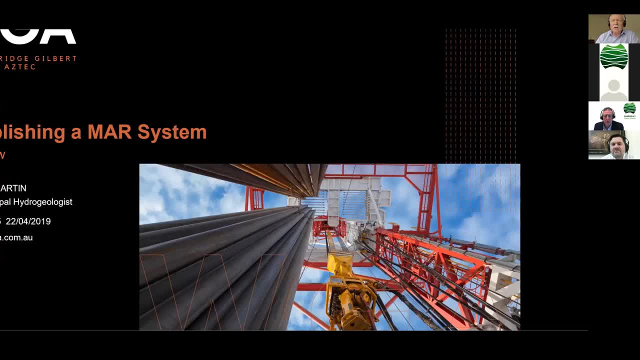 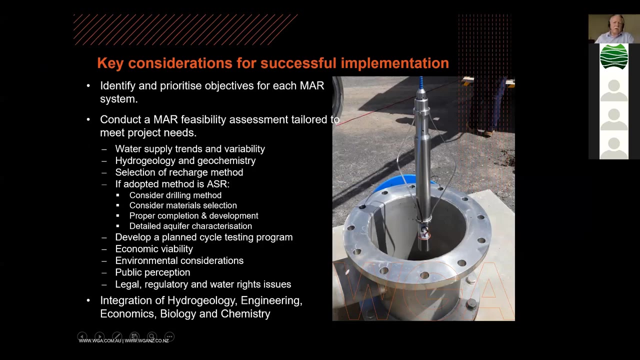 So what I'll do is I'll just through the next 10 minutes is really just cover some of the key points around delivering a managed aquifer recharge scheme And we'll take a few questions. One of the first key considerations is really identify and prioritize the objectives. 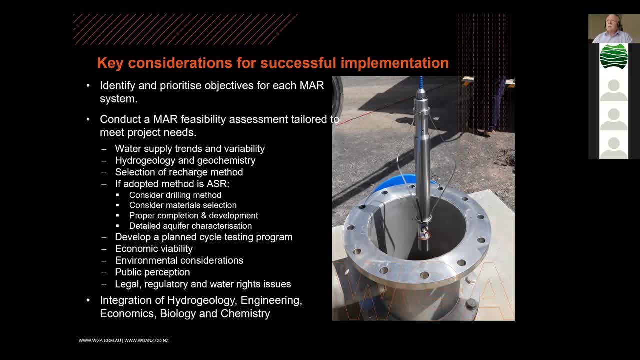 For each MAR system. Now, this is fairly important because you really want to be able to have a clear understanding of why you're actually doing MAR, And Peter mentioned four or five key reasons why you would actually undertake managed aquifer recharge. Is it for water security? 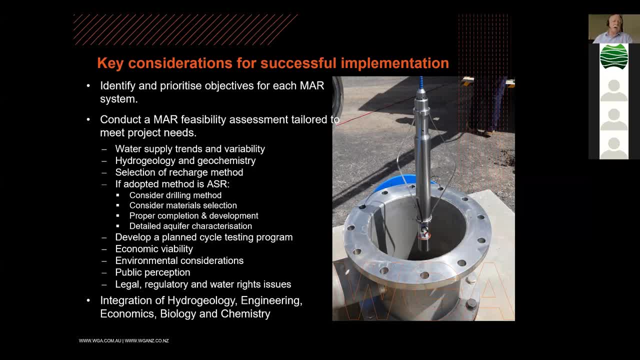 Is it for water banking, future supplies, restoration of depleted aquifers, etc. So it's really you really have to have a clear objective as to why you want to undertake MAR, And the next step is really to conduct a feasibility assessment tailored to meet the project needs. 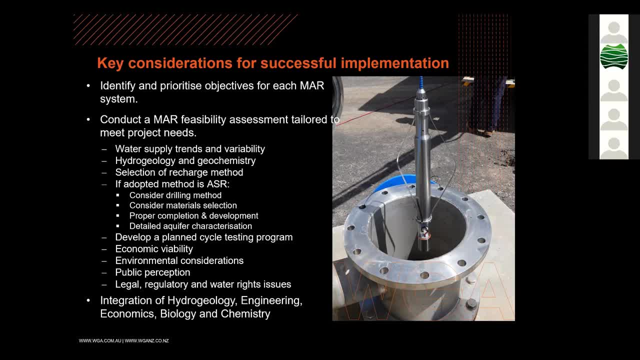 And that can include you have to understand the water supply trends and the variability in those trends. Using treated wastewater, it's available all year round, but at some times of the year there may be an influx of people into a particular area. 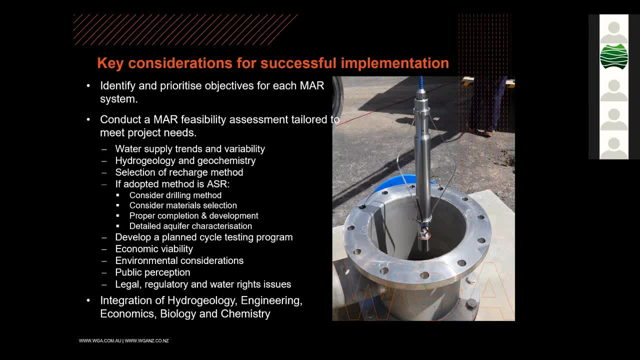 Island hydrogeology, for example, suffers from this. If you're using stormwater, it's available during the wet season, not so much in the summer. So understanding those source water supply trends and the variability in source water is actually a key. 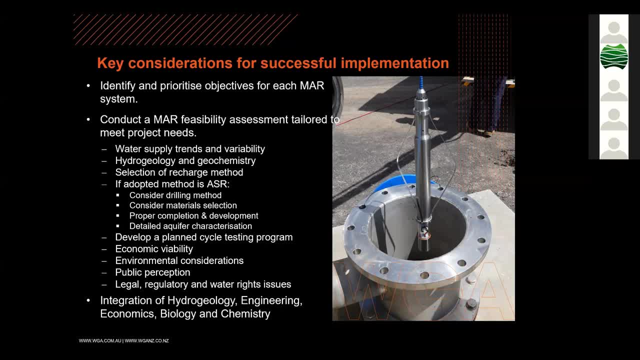 Understanding the hydrogeology of the target aquifer and the geochemistry of the source and receiving waters is critical. And if the adopted method is aquifer storage and recovery, you've got to consider the drilling method, the materials that you're going to construct the well out of proper completion and development, and detailed aquifer characterization. 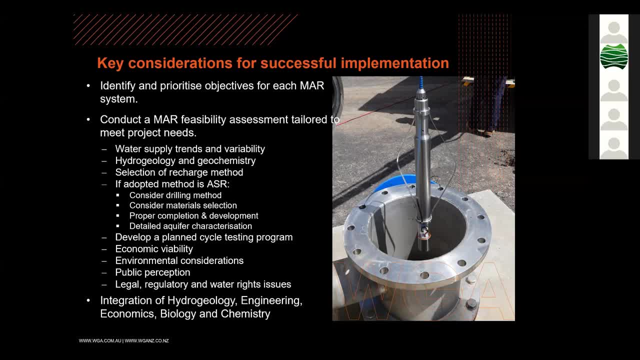 You have to understand the environmental considerations In the framework with which you're operating and certainly understanding the economic viability of managed aquifer recharge. From our experience, schemes under about 120 million litres per annum, compared to traditional water supplies, are not usually viable. 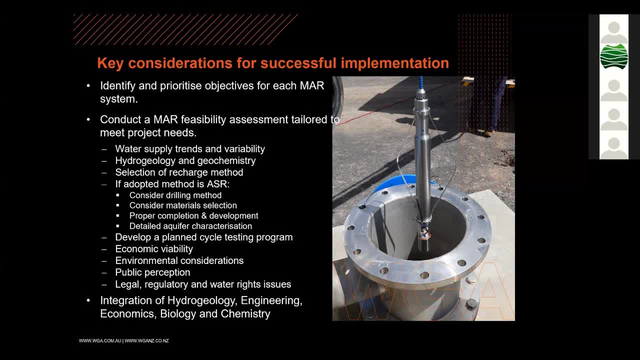 So you really want to be looking at large scale water supply. The legal, the regulatory and the water rights issues are absolutely critical to understand And we've got to remember that managed aquifer recharge is a very important part of the project And managed aquifer recharge is really the integration of hydrogeology, engineering, economics, biology and chemistry. 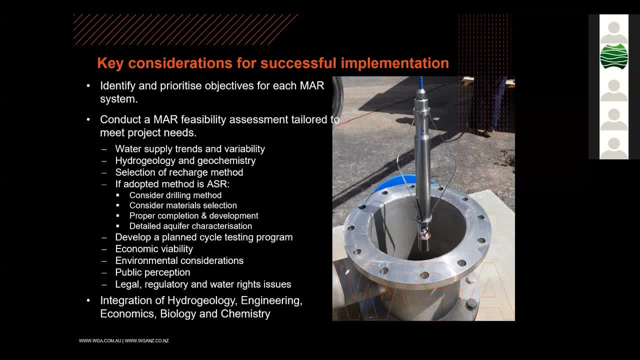 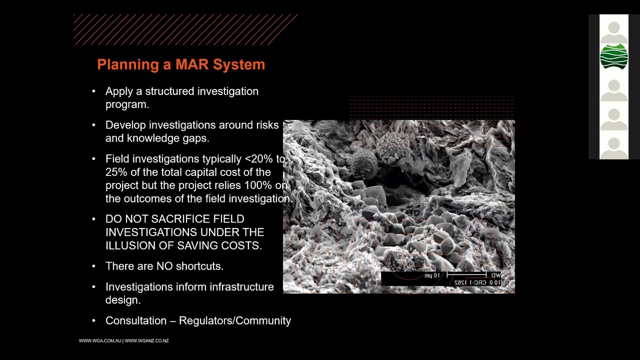 It requires a multidisciplinary approach to actually deliver one of these complex schemes And if we're not looking at bringing the appropriate teams on board, you can actually miss out some critical steps and come unstuck very easily. So, planning a MARS system, apply a structured investigation program. develop the investigations around the risks and the knowledge gaps. 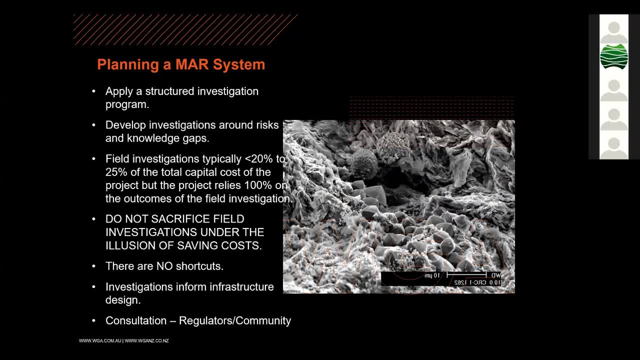 And we'll talk more about some of the risks involved in managing an aquifer recharge Field investigations- typically 20% to 25% of the total capital cost of the project, But the project relies 100% on the outcomes of the field investigation. 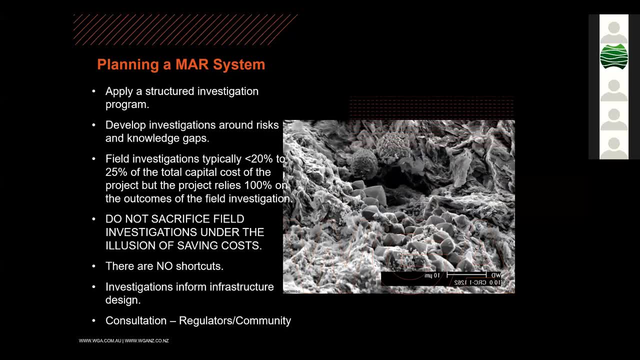 Aquifers are notoriously heterogeneous and we really do have to understand them and characterize them properly if we want our MARS system to successfully operate. And that doesn't matter whether you're doing an infiltration, basin a and or a aquifer storage and recovery. well, 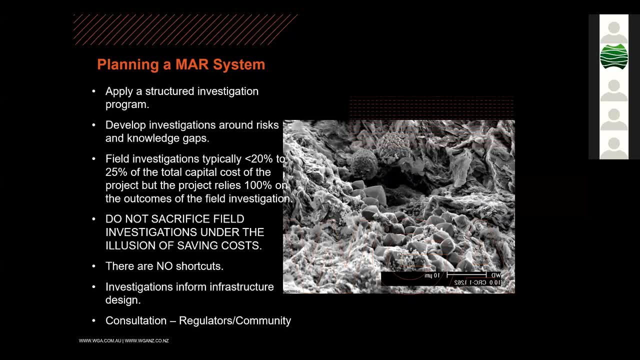 So basically, don't sacrifice field investigations and the illusion of saving costs. Those field investigations are absolutely critical to planning how you will operate the scheme Now. there's no shortcuts in taking a managed aquifer recharge scheme And quite often where I've seen shortcuts taken, invariably it's to the detriment of the project and requires a lot of rehabilitation works. 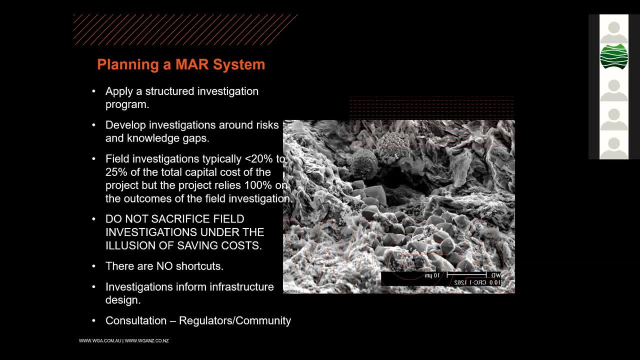 And a lot of ongoing investment to actually get it to where it needs to be in order for the system to operate sustainably. The investigations into the aquifer characteristics, the source water quality- they all inform the infrastructure design And we've got to remember that we have to consult with regulators and the community when we're implementing one of these things. 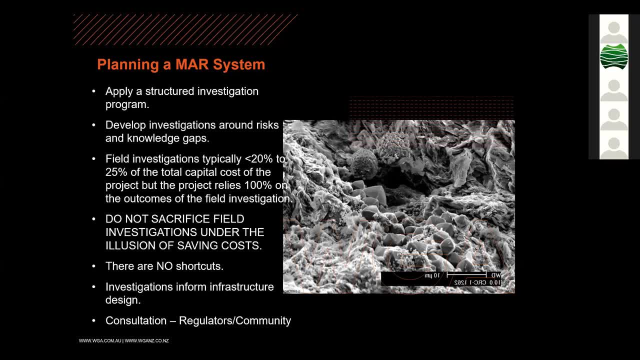 Because quite often, if we're doing it within the built environs, we're doing it on the community's back door. there's going to be lots of issues that we'll have to manage and community expectations that we'll have to manage, And so we really want to bring them along the journey of developing these schemes. 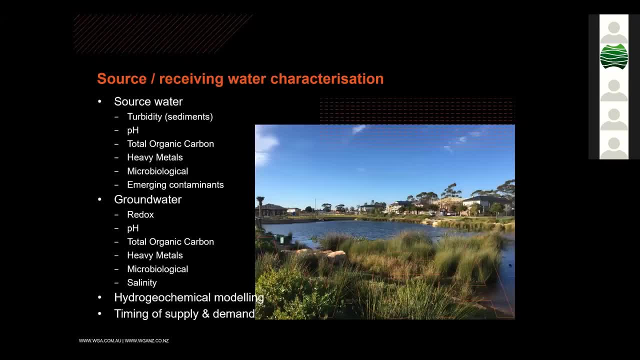 Source and receiving water characterization is probably one of the first things that we need to look at. Despite from the demand management, or when is that source water available? We need to look at some of the physiochemical characteristics of the water: Turbidity, the pH, total organic carbon, the heavy metals, the microbiological 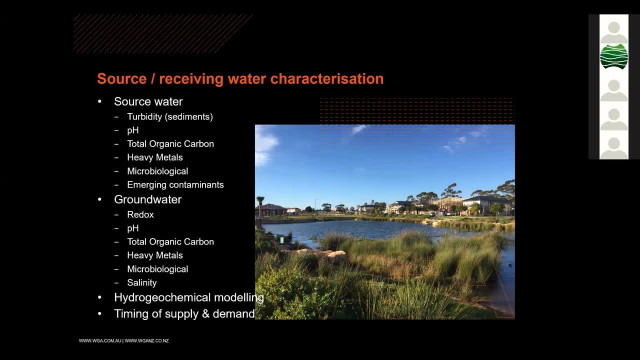 and also we need to consider potential emerging contaminants within a catchment. If we miss out on some of those, we might spend an awful lot of money only to find out that we've got a serious contaminant within the catchment that you need to manage. 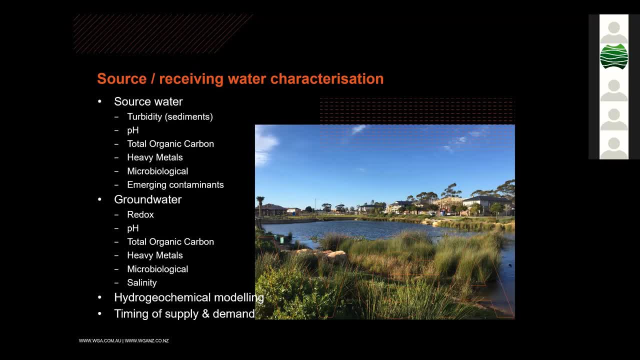 So really understanding source water quality and your catchment is absolutely critical. Now groundwater: we have to understand the redox potential, the pH, total organic carbon- again heavy metals, microbiological potential, conditions and the salinity of the groundwater system. 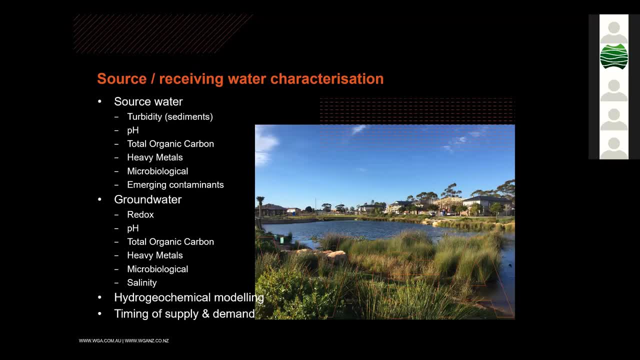 I mean here in Australia a lot of the Managed Aquifer Recharge schemes actually target brackish aquifers. Other parts of the world- the US, South Africa, etc. they're targeting potable groundwater systems But a salinity. if you're targeting a brackish aquifer, it requires a slightly different. 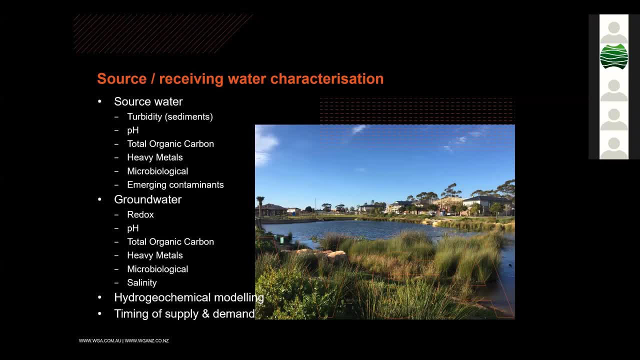 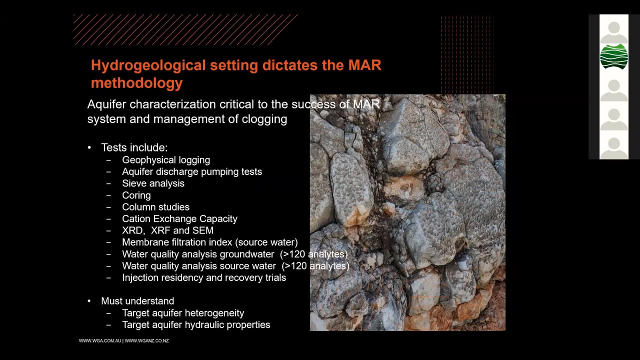 approach to the investigations than perhaps, and certainly the recovery perhaps a potable groundwater system would require. We need to do hydrogeochemical modelling and I've already mentioned understanding the timing of supply and demand of the source water. Now the hydrogeological setting dictates the Managed Aquifer Recharge methodology. 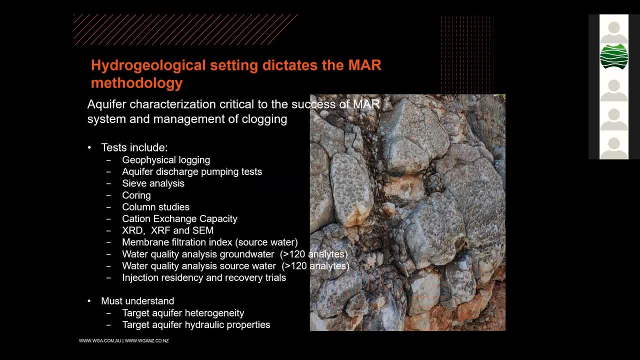 There's probably about 14 or 15 different methods of getting water into the ground. Peter touched on a number of them on the diagram from Ian Gale. But really understanding and characterising the aquifer is the success of a Managed Aquifer Recharge system. 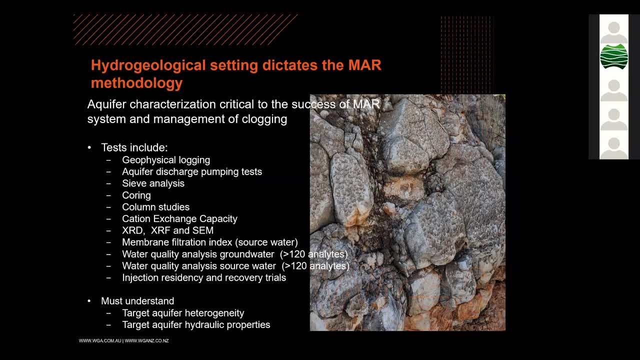 And it goes a long way to setting up how you're actually going to manage the potential risk of clogging. Now. the typical tests include geophysical logging, sieve analysis, column studies, membrane filtration index on your source water. water quality analysis of your source water. 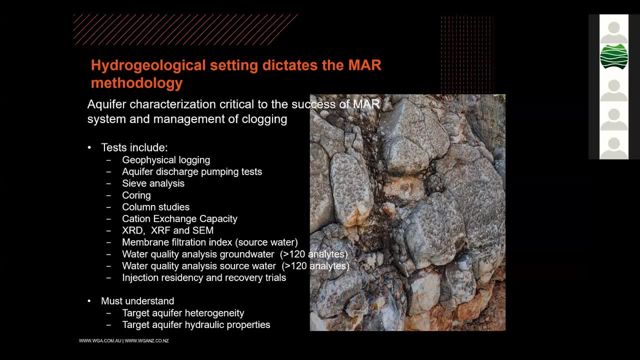 And injection, residency and recovery trials, Just to mention a few of the tests, Doesn't mean you need to do the shopping list in every single aquifer setting, but we also must understand the aquifer heterogeneity and the aquifer hydraulic properties. And one thing I haven't actually put up here either is that we also need to perhaps understand the socio-economic 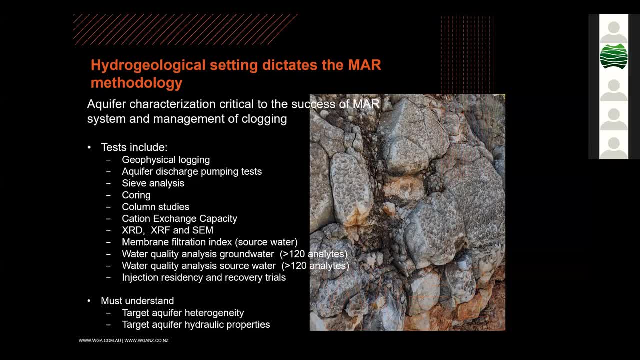 environment in which we're proposing to put a Managed Aquifer Recharge system, For example. a really, really expensive scheme with lots of water, lots of supervisory control and a lot of automation may not be particularly appropriate to be set in the midst of. 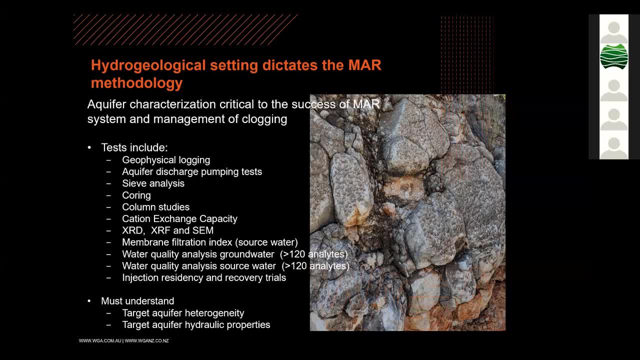 in the wilds of Africa, for example, where if a system breaks down it's going to take six to ten months to actually get the part to replace it. So you really also need to think about the capacity of the system to actually operate within those sorts of environments. 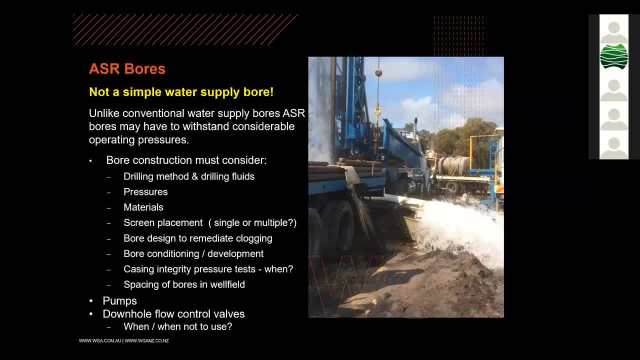 If we're talking about a man-made aquifer, if we're talking about ASR bores, one of the things I see so often and as a reason for schemes not performing is that everybody just thinks that they're a simple water supply bore. 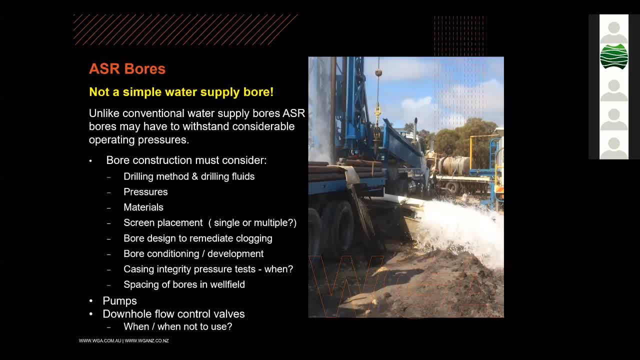 and they go ahead and construct it as they would. a simple water supply bore. It's not Unlike conventional water supply bores. an ASR bore may have to withstand considerable operating pressures. So the design you come up with, the materials you use. 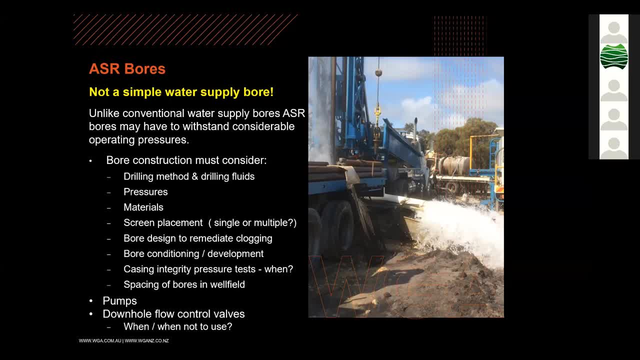 they're absolutely critical. Now, if you're constructing a bore, you really have to consider the drilling methods and drilling fluids. What sort of pressures is this system going to be operating under? What are the materials I use? And that means that you can use typically inert materials- PVC, casing, fiberglass, reinforced plastic or stainless steel. 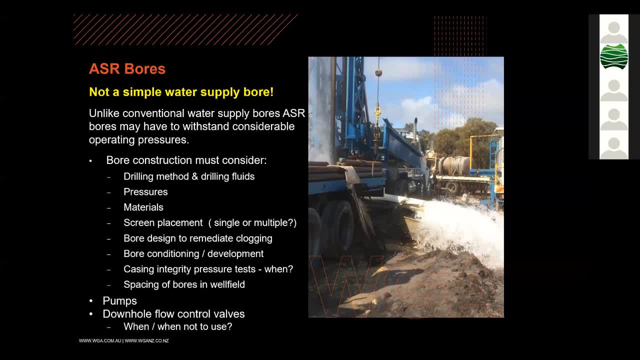 Where are you going to put the screen through the aquifer? Are you going to have multiple screens or are you only going to screen over a single interval? What's your bore design going to be like in order to remediate clogging If you use particular types of casing? are you going to actually have to undertake a pressure integrity test? 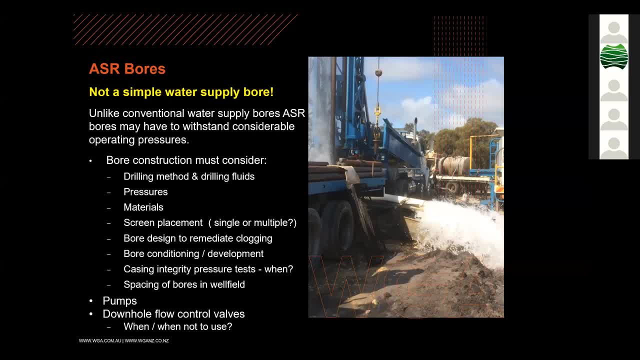 to make sure that your casing isn't going to collapse, Undertaking cement bond logs to make sure that you've got sufficient cement around the annulus if the bore is going to be under pressure. What's the optimum spacing of the bores in a well field? 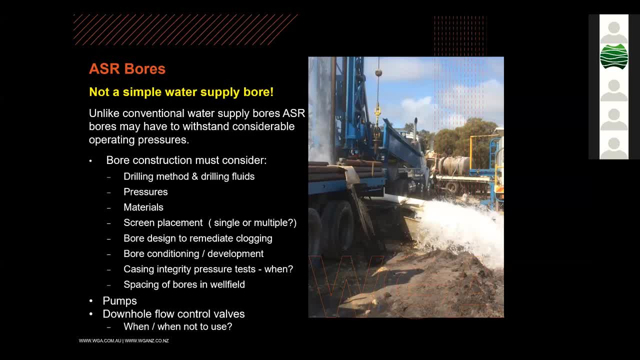 Because you're going to have just like a pumping bore during injection. if you've got a lot of high pressure heads, you're going to have interference between those bores and if you don't space them correctly you'll have a lot of interference. 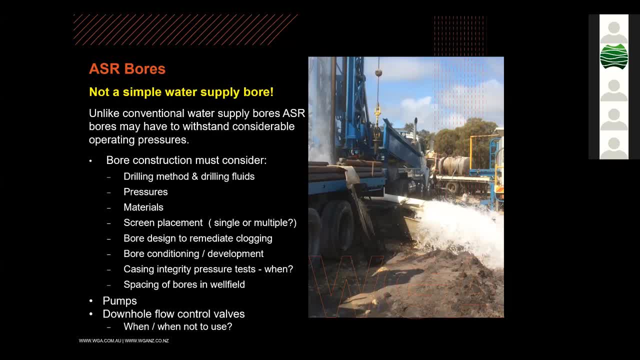 and you may impact on the capacity of the scheme to actually operate to its full efficiency. Selection of pumps is critical because we're starting often with a very, very high head above ground level and we may well be off the pump curves. Do you need to use a downhole control flow valve? 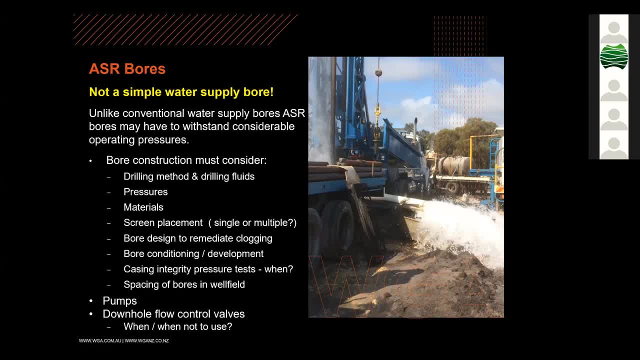 The valves are relatively expensive. They don't come cheap, and so do you, or don't you need that incorporated into the system Because it's an expensive piece of kit. it adds significantly to the capital cost of the overall scheme. The engineering design- absolutely critical to understand. 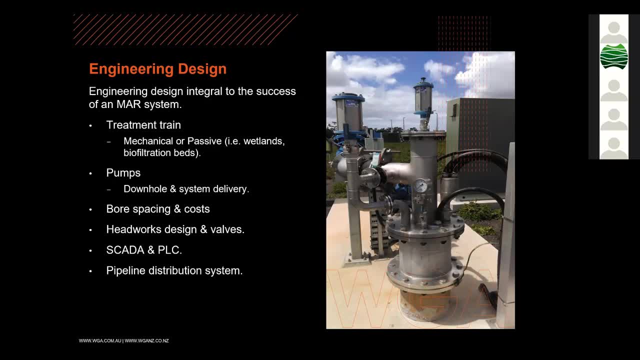 There's a number of schemes where the engineering component hasn't been installed as well as it should have, and this is integral to the success of any mass scheme. What's the sort of treatment training you're going to use? mechanical or passive Wetlands or biofiltration beds are examples of passive treatment to achieve the desired water quality before re-injection. 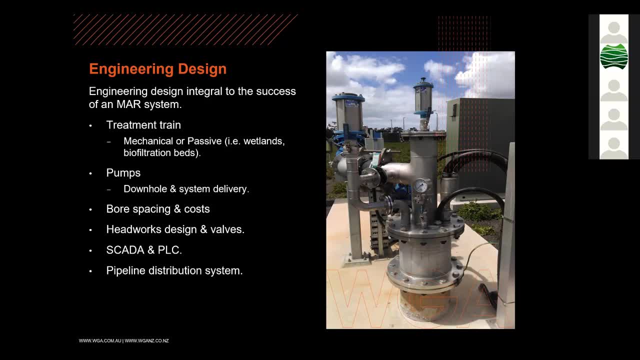 Pumps downhole, plus system delivery, both system delivery from the source and then also system delivery for distribution, Bore spacing and costs. the further apart the bores are, the more it costs to actually run cables and other infrastructure to the bores. so that's why it's absolutely critical to get the optimisation. 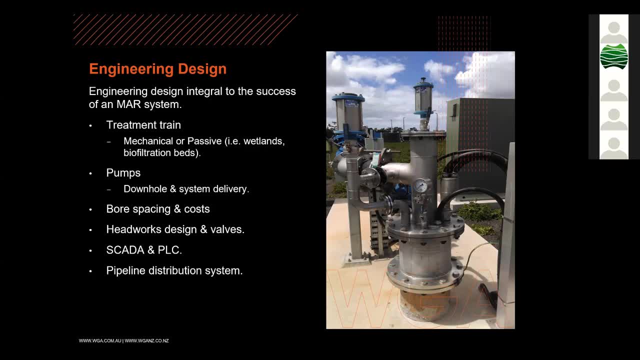 Headworks design Involving How automated do you want the actual system to be? And by automation you can actually have the supervisory control, data acquisition and the process logic control. All needs to be talking to each other appropriately so that the system can be operated effectively remotely. 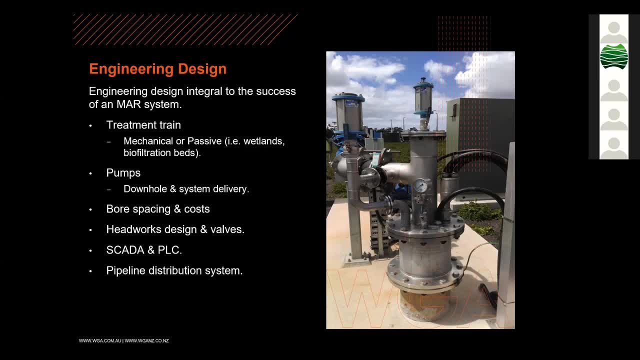 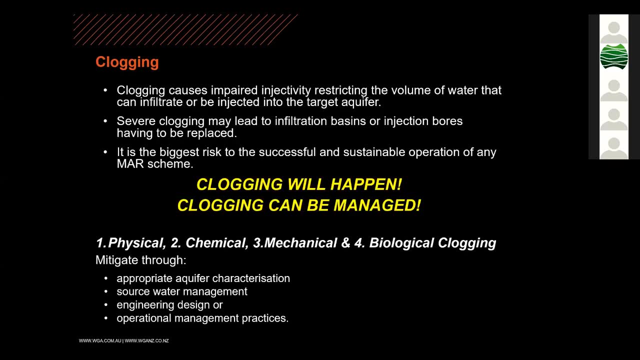 Your pipeline distribution system. how is that going to be installed and where does it need to go to actually meet demand? Clogging is the last little topic I'll actually touch on. Clogging causes the impaired injectivity, restricting the volume of water that can infiltrate or be injected into a target aquifer. 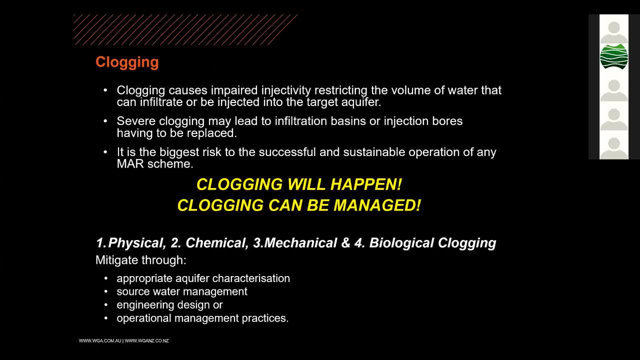 Now, severe clogging may actually lead to infiltration basins or injection bores having to be replaced, and it's the single biggest risk to the successful and sustainable operation of any mass scheme, And that's absolutely critical. as to characterisation of the aquifer, because that will determine how we actually then construct. 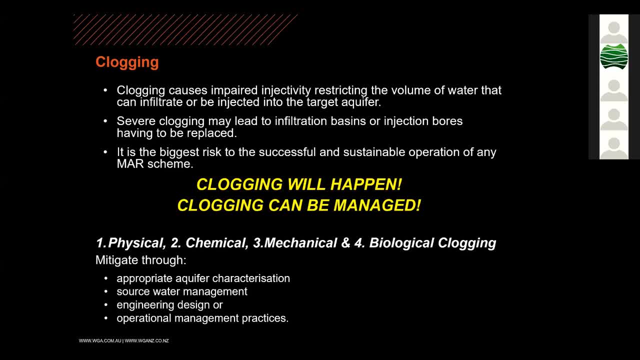 our mass scheme or the most appropriate mass scheme we might apply for that hydrogeological environment Clogging will happen, but the good news is that it actually can be managed. The question is: do you manage it through infrastructure and as part of the treatment train process? 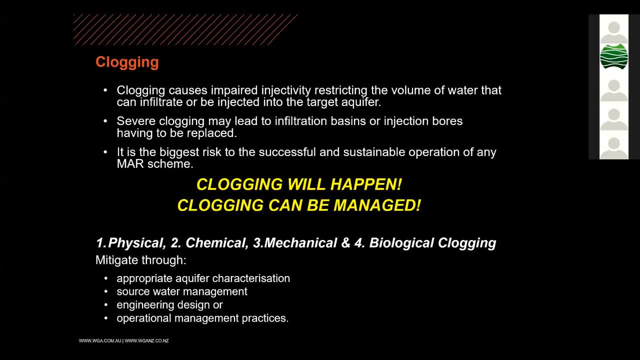 or do you manage it as part of your operational aspect? There's four key contributors to clogging. You can have physical clogging, which is typically drilling muds, Chemical clogging, associated with precipitation of iron or aluminium silicates in the well bore, or even calcite. 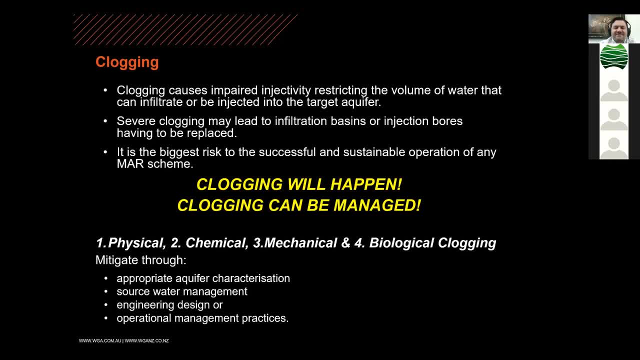 Mechanical clogging often occurs during the drilling process, where drilling muds haven't been adequately removed from the well or there's been insufficient development of the bore prior to drilling. Biological clogging: All aquifers have a unique microbiological system and most of the little bugs secreted 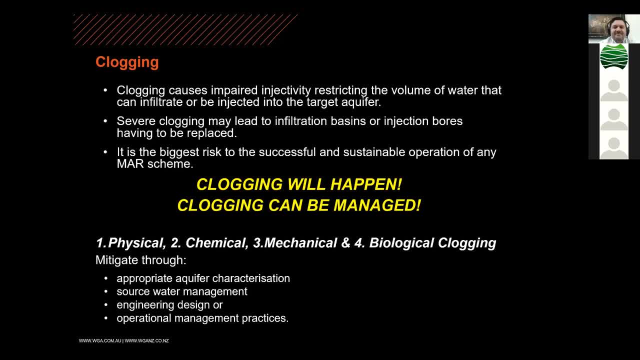 treat slimes and that's what can cause clogging. So if we haven't managed our water quality right and we haven't got that balance right, we can actually facilitate good conditions for those bugs to actually grow and they will cause clogging. Now, as I mentioned, we can actually mitigate clogging through appropriate aquifer characterisation. 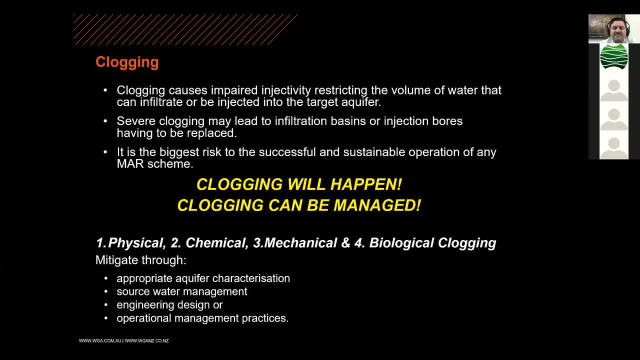 source water management, engineering, design or operational management practices, And I'll talk more about clogging and system design work in a bit. We've got a lot of work in the online seminars, online courses that are actually coming up in July and October. 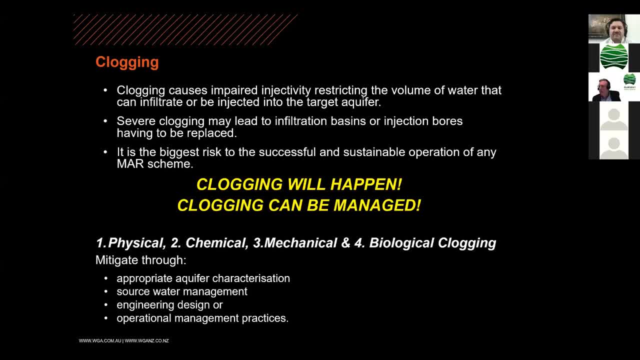 But I think that's about it from me, unless there's any immediate questions somebody wants. That's excellent, Russ, and it's covered a lot of ground again in a short space of time and I can realise more and more how much these courses, online courses- you just mentioned- 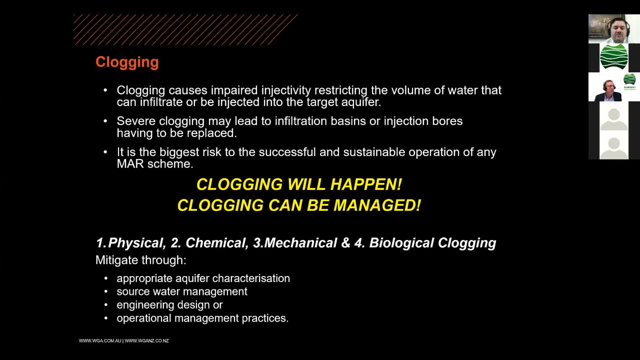 are going to be important to many up in July and August. Maybe we can just take this one question from Rob Richardson at HydroDisc. That might be useful if you're there, Declan. Rob Richardson from HydroDisc has said: how is the extraction of water from the receiving aquifer by private corporate bulls managed, slash, controlled? 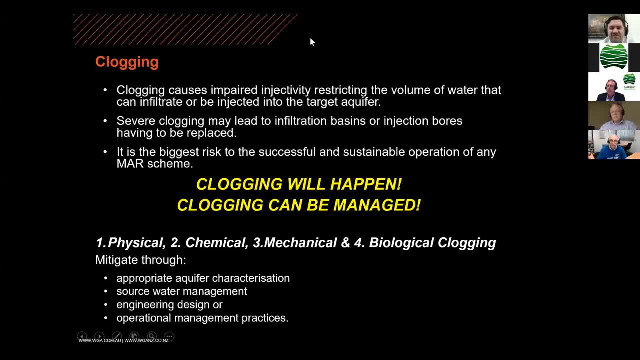 Well, here in South Australia, for example, they would have a licence typically to extract a certain amount. How is it controlled? It would be controlled by the method of the pump and the engineering. Russ will probably talk to that. Yeah, the control of the extraction, certainly, as Declan mentioned. 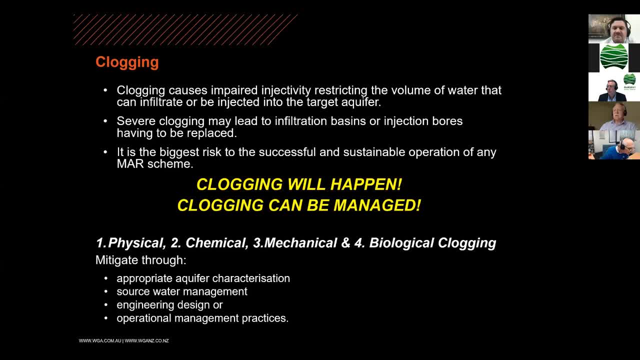 it's licensed in South Australia and licensed through many places in Australia, So the operators have a licence to recharge and a licence to extract And the pump set up and design is geared to manage the maximum heads that you might experience during injection And also the maximum drawdown that you might experience during injection. 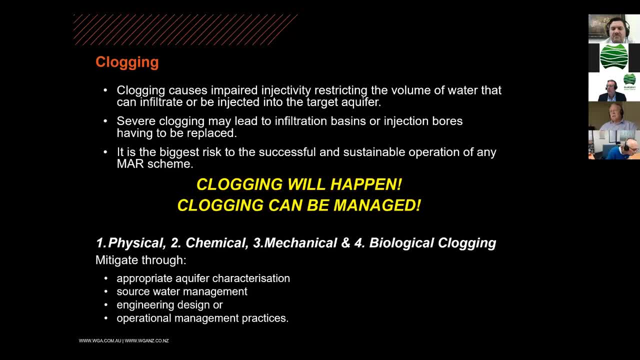 And a lot of investigation goes into assessing the potential risks associated with the Managed Aquifer Recharge Scheme on existing users. and where existing users may be impacted as a result of the Managed Aquifer Recharge Scheme, There are mechanisms in place that need to be implemented to make sure that those existing bulls aren't going to be adversely impacted as a result of the Managed Aquifer Recharge activities. 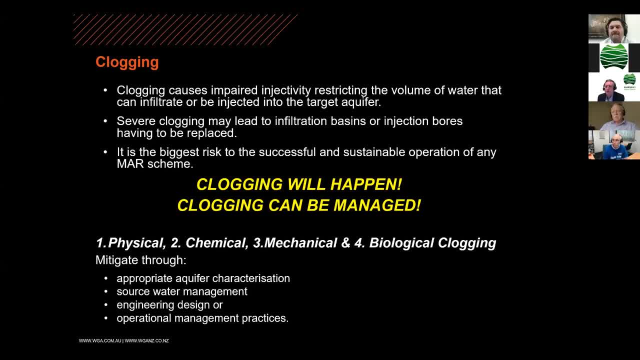 Yep, that's great. So, Peter, any comment from yourself on that question for us. That question from Rob: how is the extraction of water managed and controlled? Have they covered it well with Russ and Declan, I think they've covered it. 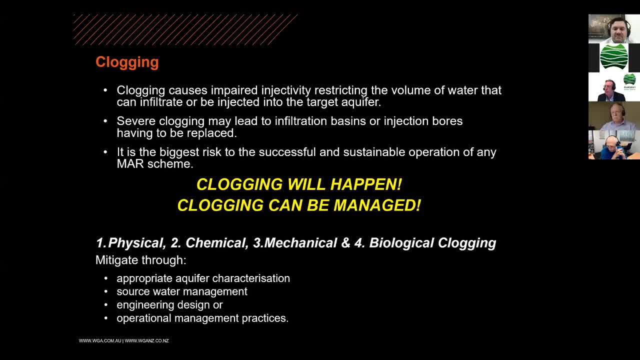 Yep, that's all right. There are differences between jurisdictions and I think there's still room for improvement in the way that entitlements are awarded Yep, But I think that's something maybe for the course Yep, for sure, Yep, that's happening quite a bit in this webinar. 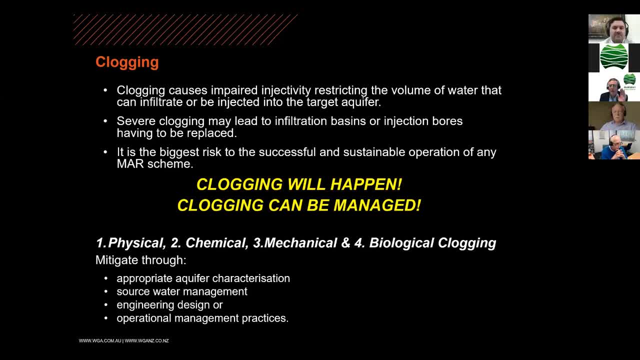 There's a lot more questions we can go to, But look, before we do that, I think it's best if we move straight on. Thanks very much, Russ. Thanks so much, Peter. We'll move straight on to Declan's presentation and hand right over to you Declan. 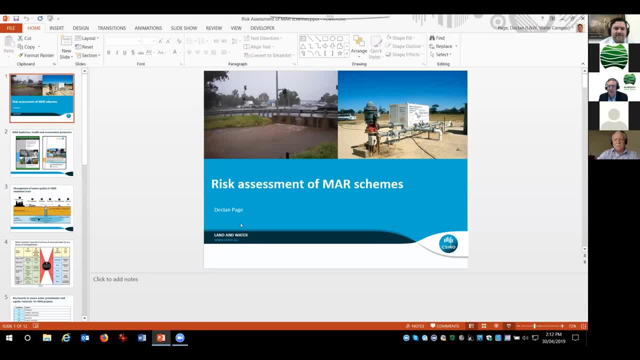 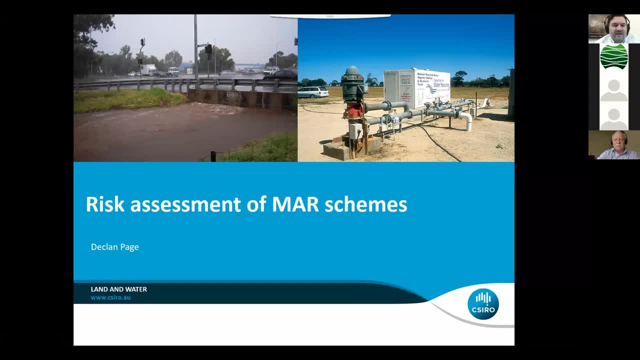 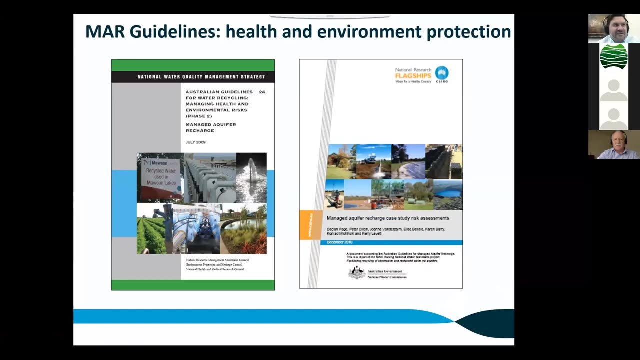 Okay, thank you. All right, Risk assessment, am I asking? I'm going to talk here about the Australian experience. Most of it happened in around 2010.. We had a large drought which really motivated, I guess, Australian governments of all natures to get MAR and get some guidance together. 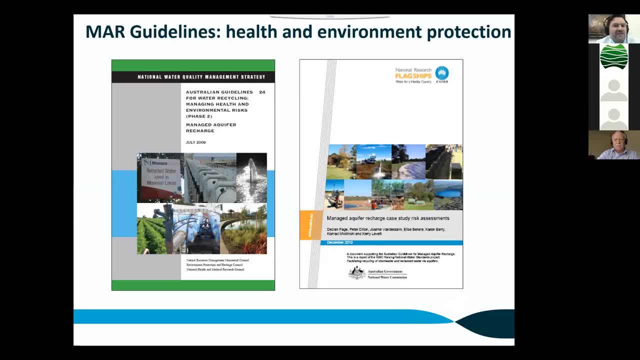 The National Water Quality Management Strategy, the Australian Guidelines for Water Recycling. They're about 10 years old now. They were developed then and there are risk-based guidelines very similar to that used by the World Health Organisation for drinking water, Also pointing to some case study risk assessments that are also put out about that time to show how it would go through the. 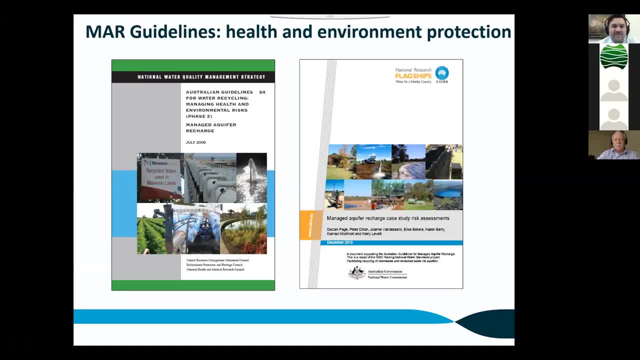 actual risk assessment process. I think they've served us quite well and I'll just give you a brief step through about how they work. Some people think they can be overly complicated, but if you use a structured approach, as Russell said, in your investigations- 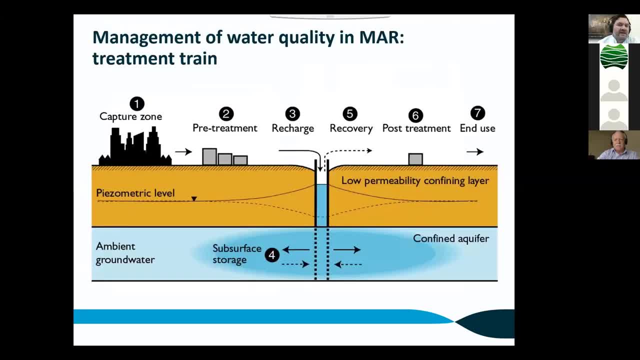 you can work through these quite easily For each MAR system, regardless, I guess, if it's stormwater or wastewater, or if it's used for drinking water or irrigation, we can specialise it in terms of these seven components being the capture zone. 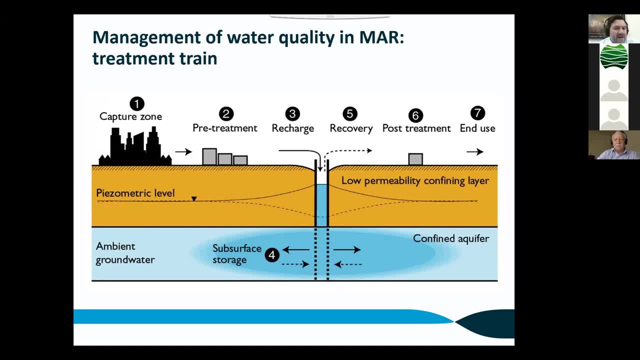 any pre-treatment that might be used some way to get the water into the aquifer, stored there for a period. it's then recovered. There might be a post-treatment required and an end use, And each of these seven, I guess, components is a component of where the risks need to be assessed. 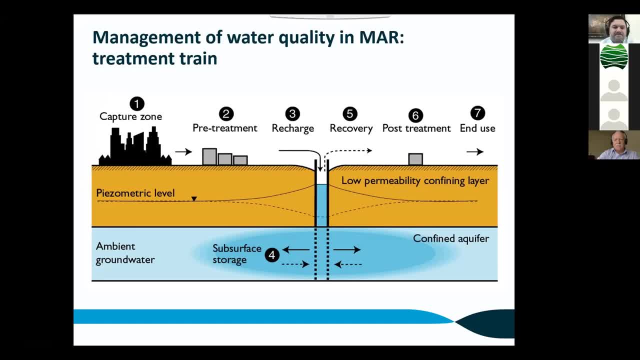 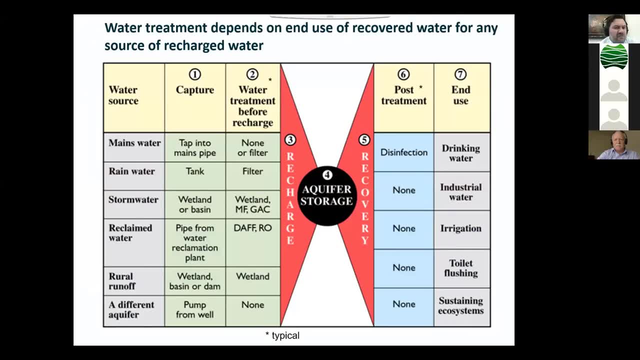 and where else are the risks and then also have the opportunity to be managed. So there's an old diagram, but I really want to get across here is: regardless of the source, water use, the type of capture zone, how much treatment you want to use. 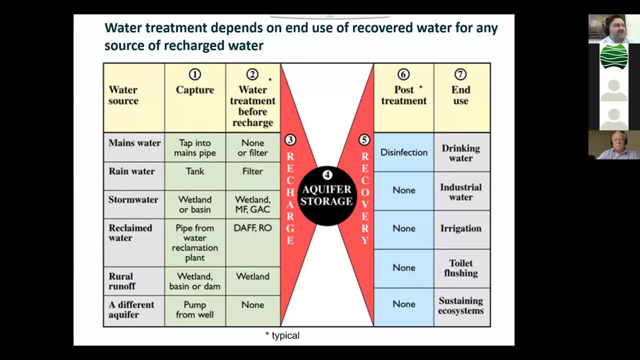 it's the aquifer, really, that integrates all these different configurations, And there are very many based from very simple systems, like Perda mentioned over in India, with check dams used for irrigation, to very, very, I guess, highly engineered, highly complicated systems. 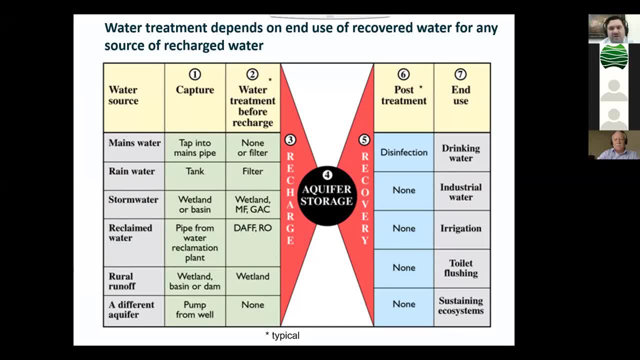 Where they're used for drinking water augmentation, like in Perth in Western Australia. But in each of these, these seven components, I guess, are consistent to all of them And understanding each of these seven components, I guess, is a treatment train. 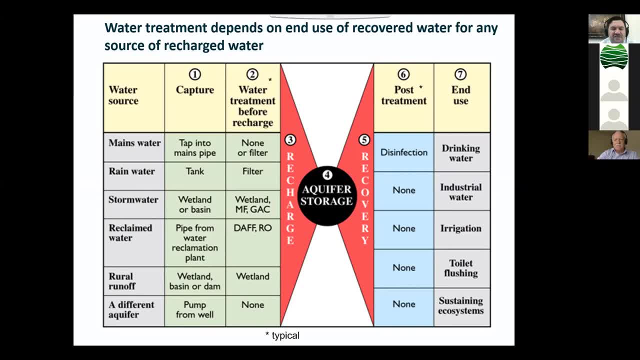 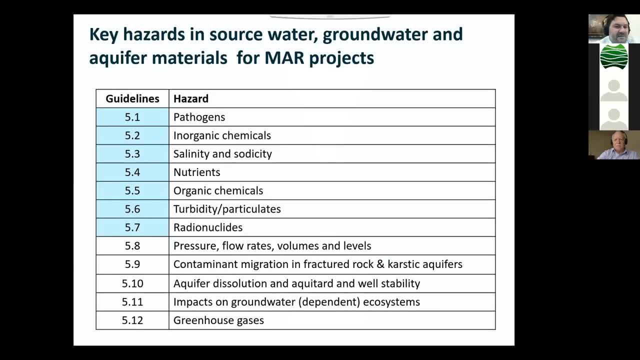 what we call barriers to manage risk is essential to the entire risk management process. So in the Australian MAR guidelines we have 12, I guess- key hazards. which hazard becomes a risk. The first seven are water quality hazards and the last five are unique to aquifers. 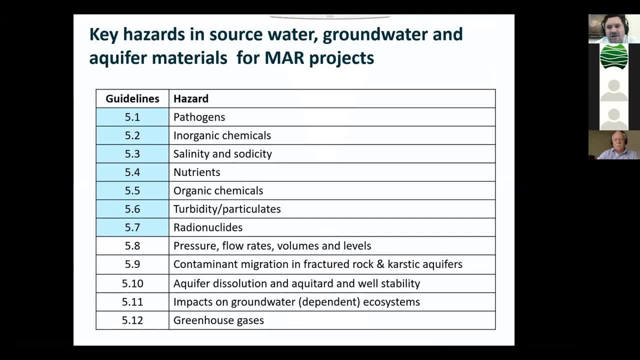 So the first seven you'll find also in things like drinking water guidelines and the like, but the last five are unique to the Australian MAR guidelines. Generally, when we manage for water quality, pathogens is probably one of our key risks. that and organic chemicals. 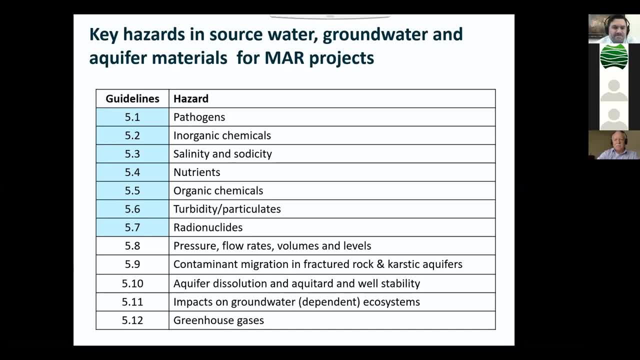 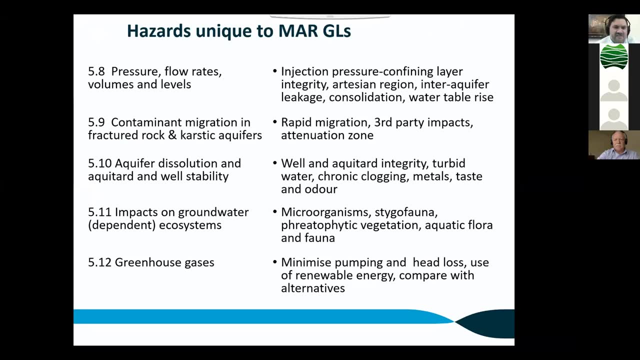 when it comes to human health. But some of these other things, other hazards, for example salinity, can be critical for things like irrigation. Anyway, the MAR guidelines are unique in that they have these last five hazards which are looked at, which aren't water quality hazards. 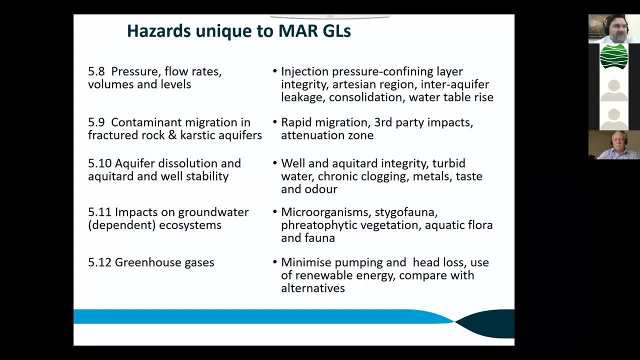 So understanding things like pressure and flow rates and volumes. So, especially, as Russ said before, if you have a cluster of MARs and you don't know the names, you may injection in one may affect the other, Understanding migration of water within the aquifer. 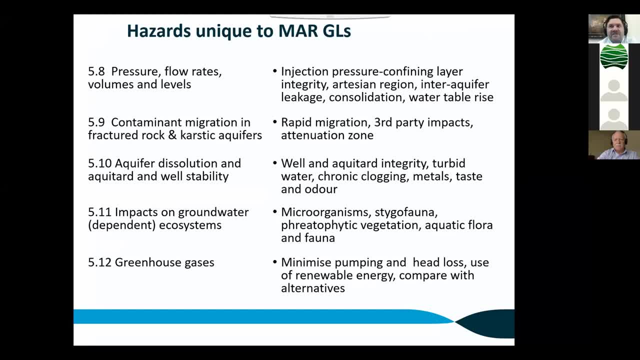 So fractured rock and caustic systems may not behave very simple And understanding where your hazards might go. they may go further than you may think. Aquifer dissolution and stability is another important ones Again for things like caustic aquifers. 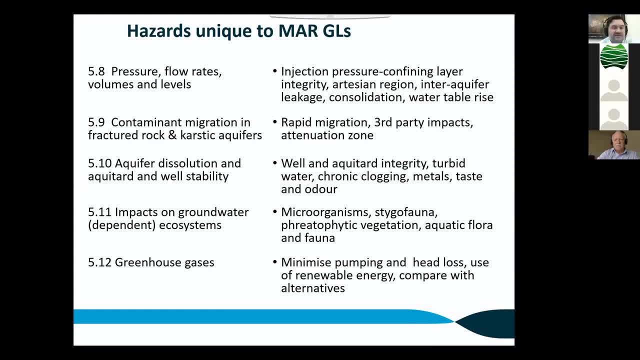 that's, limestone aquifers, if you're to inject things like stormwater, which is commonly done here in Adelaide and it's slightly acidic and will slowly dissolve. the limestone can be a good thing, though, because it can offset some of the effects like clogging. 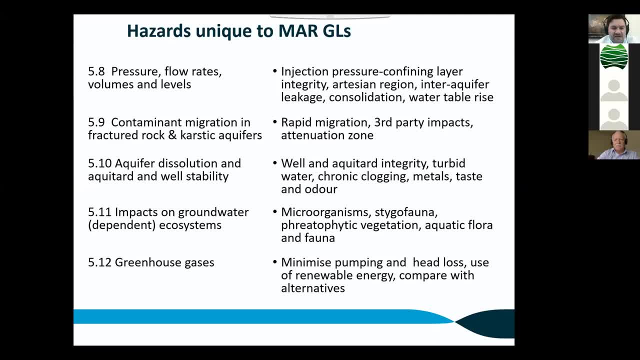 that Russ described before. Lastly- second to lastly- is impacts on groundwater systems. So you know, water that you inject may have an impact or cause either flooding to a local groundwater system. It may completely change that ecosystem and that needs to be taken into account. 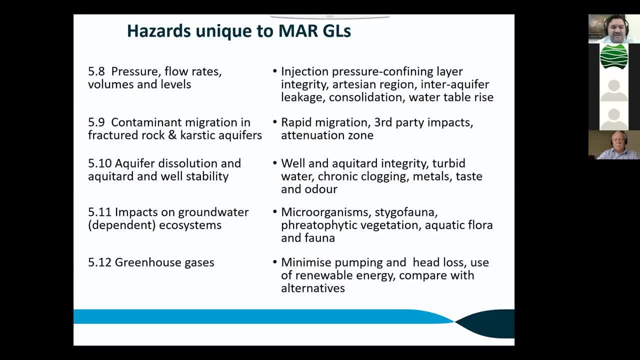 And lastly, greenhouse gases. I guess this was an attempt here to realize that you know. greenhouse gases affect the planet as a whole And we don't really want to be recommending water supply options that are more energy intensive than others. So I guess at its simplest. 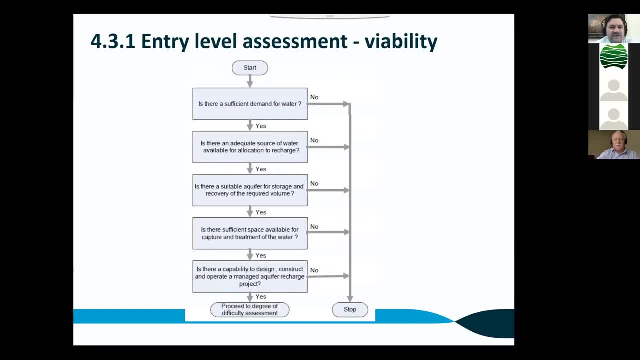 this is what's called an entry level assessment. it's a viability assessment. It really just takes you through this. yes, no diagram. These are straight from the Australian guidelines And I'd ask anyone to look at those as a first starting point. 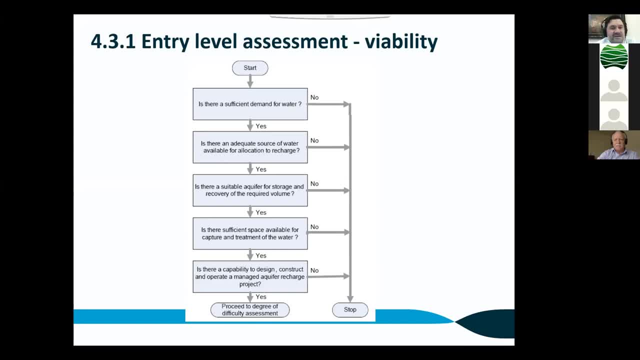 But really it just asks: is there water to be recharged, Is there somewhere to recharge it, Is there a use for that water And is there a capability to manage that entire system? And if you've got yes to all those things, 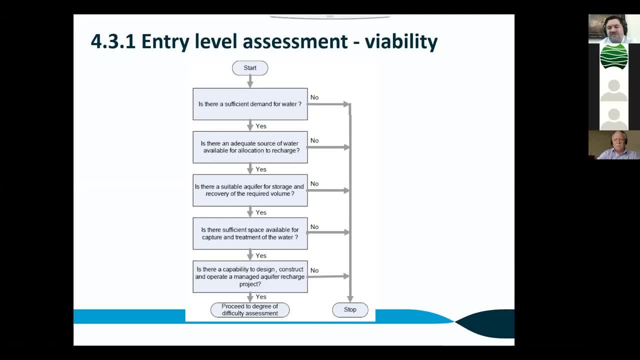 then I guess you've probably got a what's at least a viable system that might be worth investigating. And too often MAR is looked at as we need a recharge. We don't really know why we want to recover it or those really simple high level questions haven't been answered. 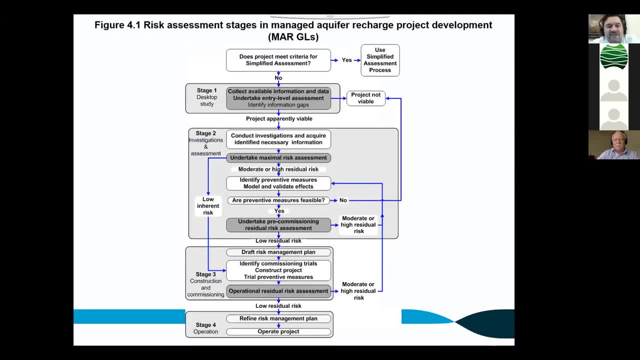 Let me go into the complicated success diagram. I don't expect anyone watching to understand all this here Just from what I'm showing now. But what I do want to get across is it's a staged approach. Starts with a desktop investigation, Then you go to field. investigations could also be laboratory studies. 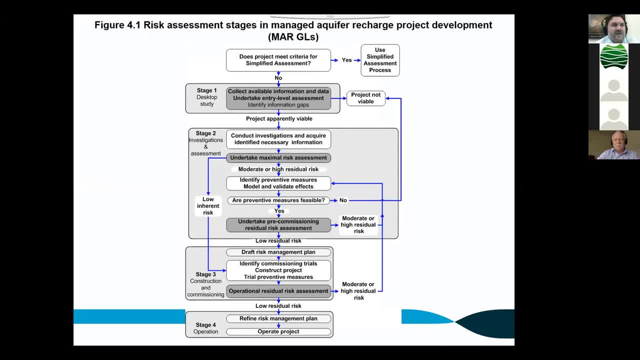 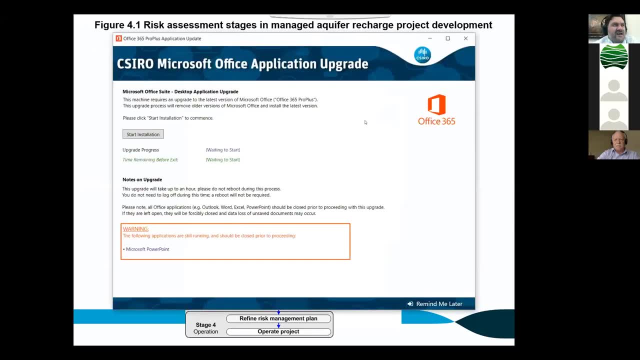 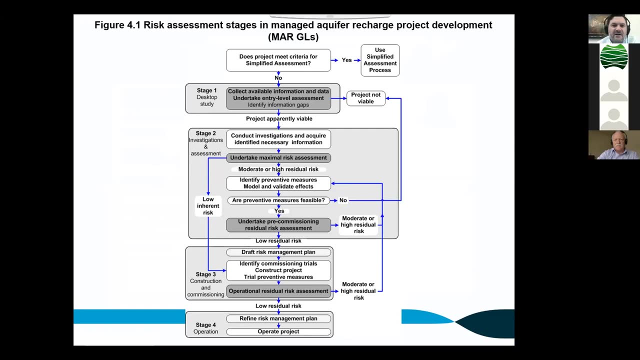 Then there's a commissioning stage with full scale testing And finally the operation stage. It's during the operations stage that you can refine and develop an operation or a risk management plan. I like to use this example here of a simplified assessment. 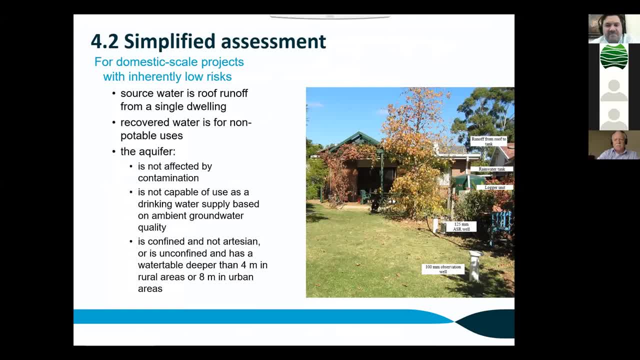 People always think: you know, these things have to be really, really MAR schemes have to be very, very complicated. This is actually Peter Dillon's backyard. We did a test there, But this takes- this is rainwater taken from a roof- 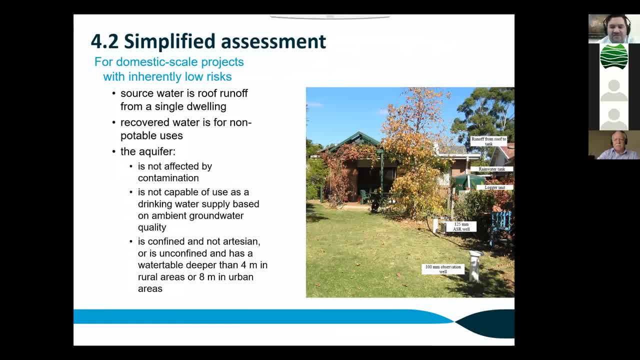 goes into a tank and into an ASR well. There's an observation well just nearby there as well. But because the risks were inherently low, it didn't need- not it didn't need- a high level of investigation in terms of water quality or in terms of 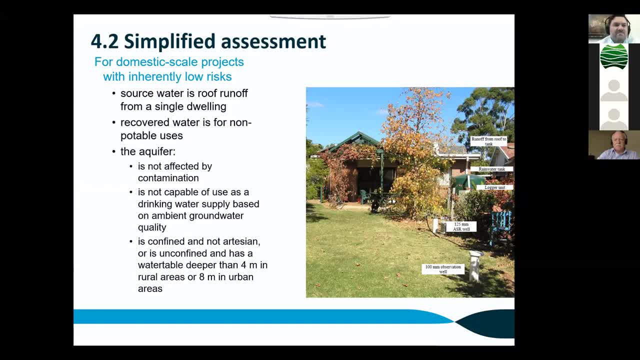 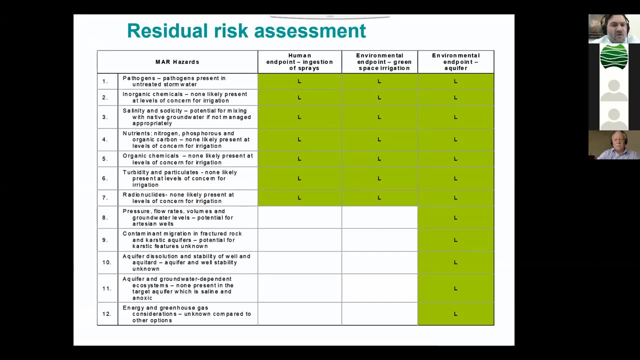 understanding the aquifer. So for a small scale system using treated rainwater in this case, a simplified, a simplified assessment was sufficient. In the end, though, I guess the way we like to a way to organise all those risks is on the first column. you've got all the different, all the different hazards. 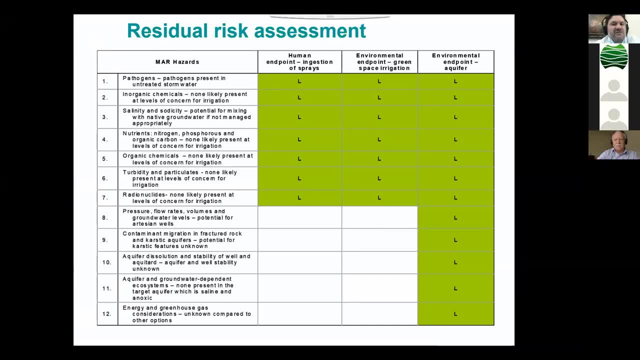 And in each of them we have, for each of these hazards, we have to look at the end point. So the risk end point might be human ingestion, It might be irrigation landscape or it could also be the aquifer. Initially, some of these might be. these are all classified low or green. 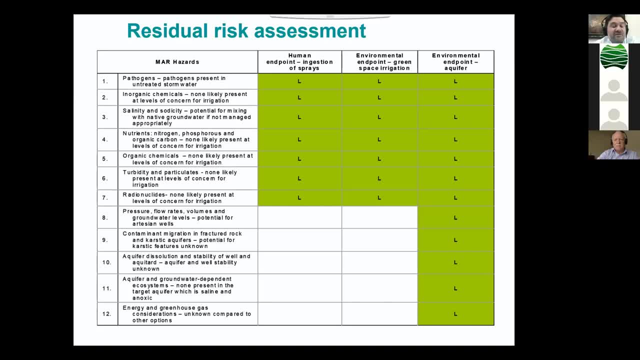 or low risk now, but they might be red. So, for example, if you had pathogens present in your storm water and you wanted to drink it, you might need to look at some sort of treatment prior to prior to drinking. Similarly, if there were organic chemicals present or nutrients, 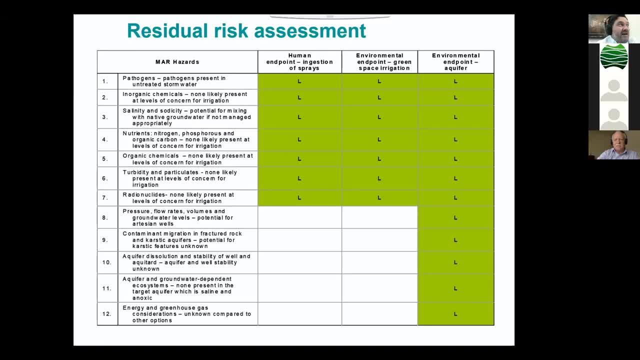 again, some sort of treatment or some or even passive treatment in the aquifer might need to be considered. But these treatments can be added or passive treatment can be measured. And once you've added all these together in that, in that train I showed 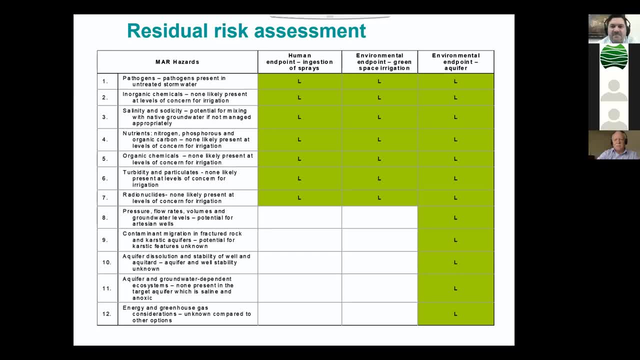 before with the seven key components of the of the MAR scheme. eventually, you want to get them all to green, like this, And again this is an example from Peter's backyard, very simple one, And so they're all green, and he was able to proceed. 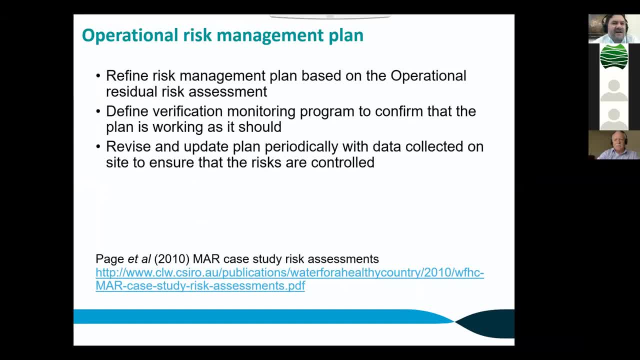 I guess the last point I want to make is that there are, since, since these have come out, there have been a number of, I guess, bigger investigations put put into place at both in Perth and Western Australia. They've got their their recharge scheme there for their drinking water. 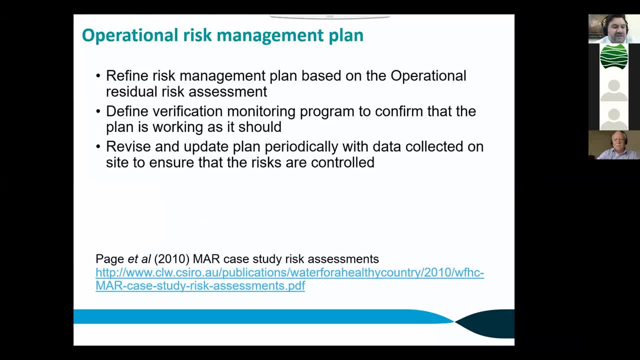 supply, but also here in South Australia the Gordian Institute recently published a series of stormwater MAR health risk assessments And I'm happy to pass on the public those publications and give links to those interested at a later time when I'm 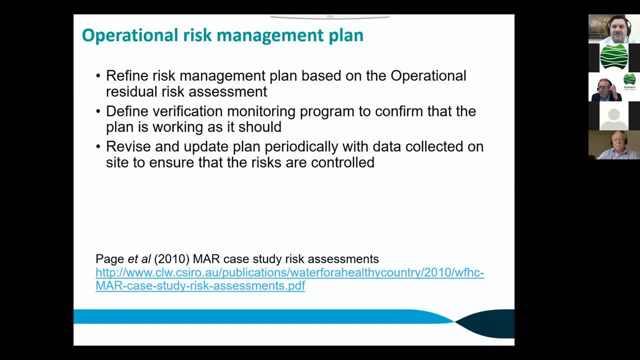 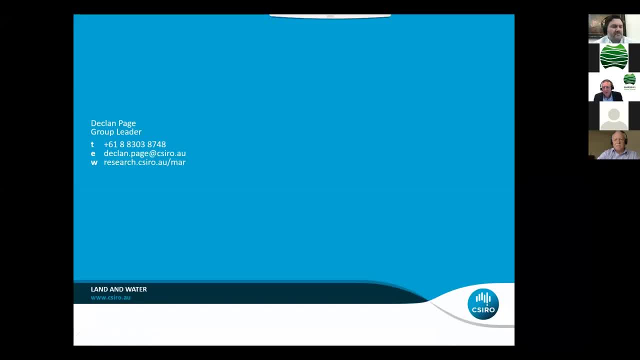 when I return to work. I think that is it for me, Thank you. Thank you, Declan, Thanks so much. It's it's it's a huge area and we're covering vast amounts at once here, but we'll we'll endeavour not to do that as time goes by. 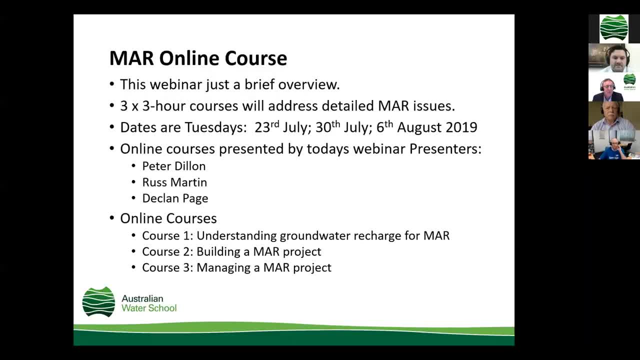 But let's start taking some questions. We've got about 10 minutes really, But let's, let's. let's look at these questions. There's some in the chat line, I notice, And there's one or two over here in an email. 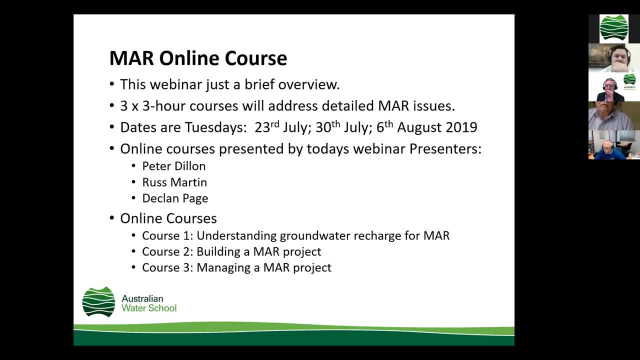 I'll. I'll come to them. Before we come to them, I just want to emphasise that the MAR online course will do what we couldn't possibly have done today, And that is that we're going to go into some detail. You can see there's a, there's a poll, just come up there. 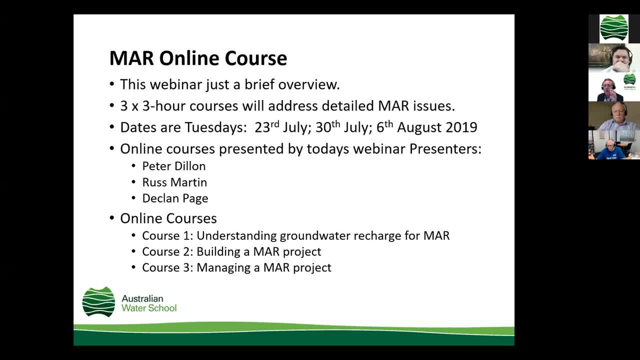 But I just wanted to make this point here. There'll be three three-hour courses online discussing the three items at the bottom of this, this slide right now: Understanding ground water, building a MAR project and managing a MAR project. The three presenters will be the ones we have here today, as you can tell. 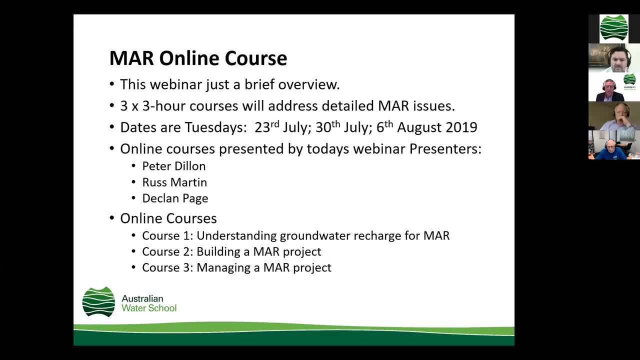 We've been doing this for decades and have covered just about everything you can cover in MAR, And so I wanted to really emphasise that. So, all right, let's go to these questions. One here from Vanessa from Land and Water Consulting. 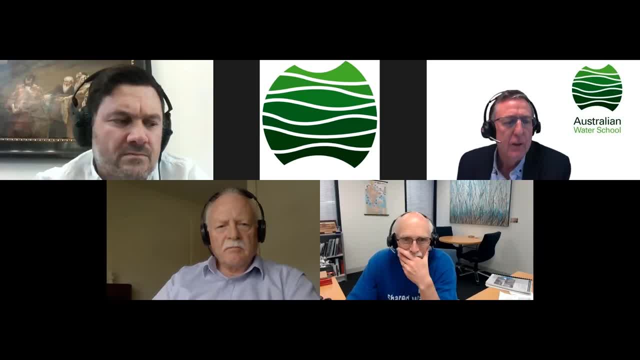 Has there been any recent instances where a targeted aquifer has become contaminated through a MAR scheme, and how was that managed? Sorry, gentlemen, Declan, Peter, Russ, you won't see this question. It's come through an email, but I'd just like to get a comment on it briefly. 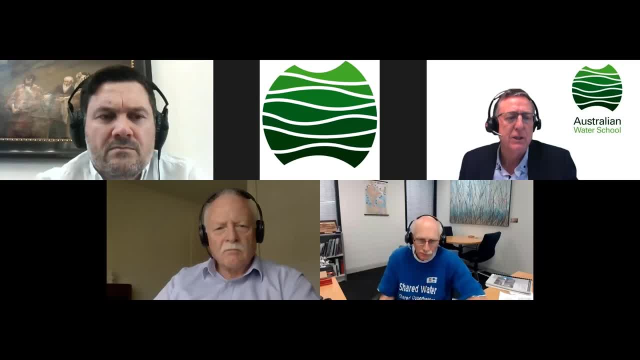 Any any recent instances where a targeted aquifer has become contaminated through a MAR scheme, and how was it managed? managed? Who wants to shoot off first? I guess I can answer that one Trevor Short answer is yes. The level of contamination is unfortunately one of these new emerging contaminants, PFAS. 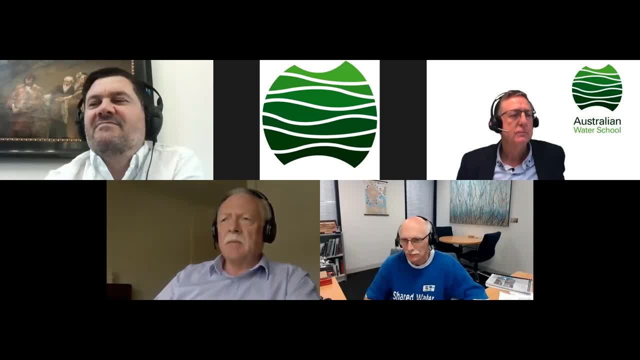 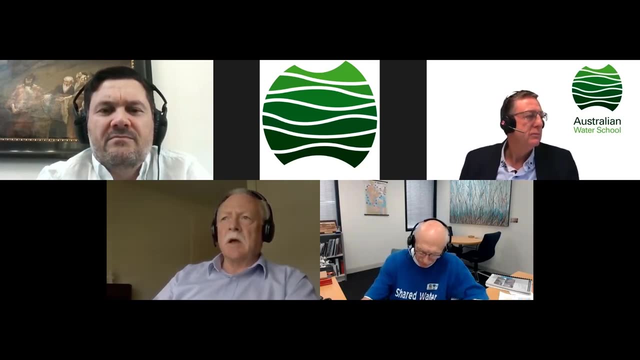 The level of contamination is actually still below the national EPA guidelines for the beneficial end use of the water And, however, the operator of the scheme has, as part of their risk mitigation strategies, shut the system down for the time being, until they resolve how and who is going to be responsible for assisting in the remediation. 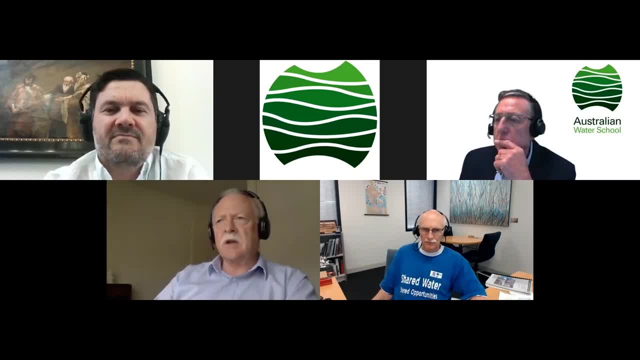 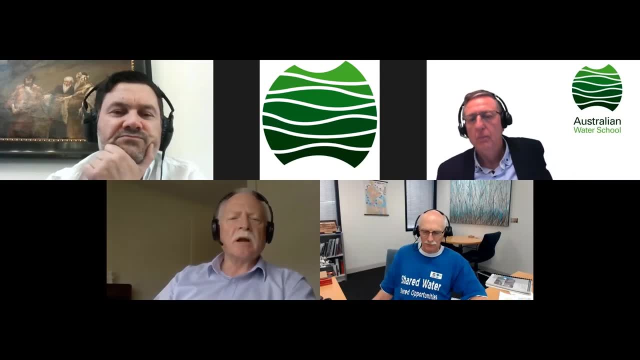 There are potential remediations and options in train, But, yeah, it's just a question of working through all of the risks, all of the issues and what it actually means. Yeah, Any comments? Declan, Your mic's not on, by the way. 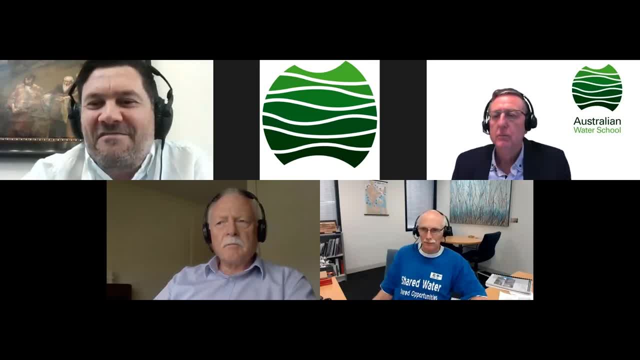 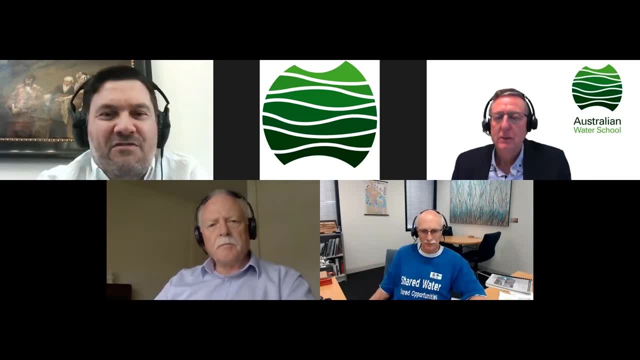 Hit your mic. Yeah, look, I thought exactly the same one, Russ. Well, I won't mention which one, but PFAS is a chemical which is present pretty well in all stormwater and all wastewater all around. So the more you look for it, the more you find it. 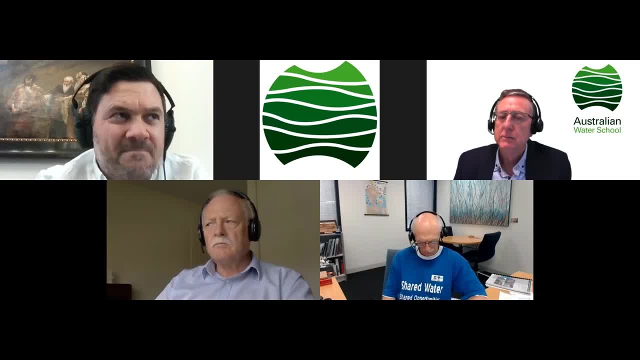 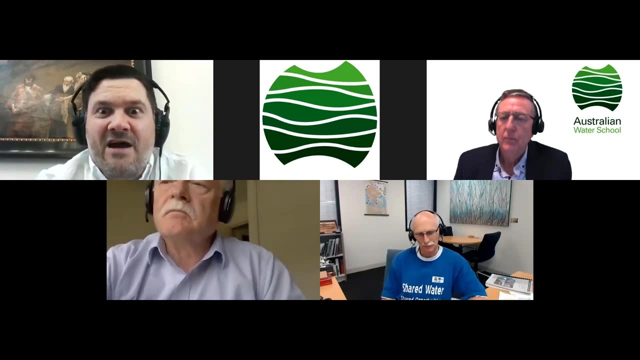 In this case, that system was shut down And, by the way, by the proponent. in terms of regulation in the future, I think there's going to be some changes in how some of these things are regulated, because they are emerging chemicals and the risks are unknown to a large degree. 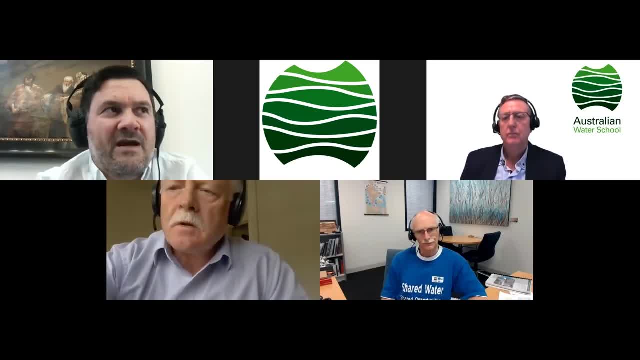 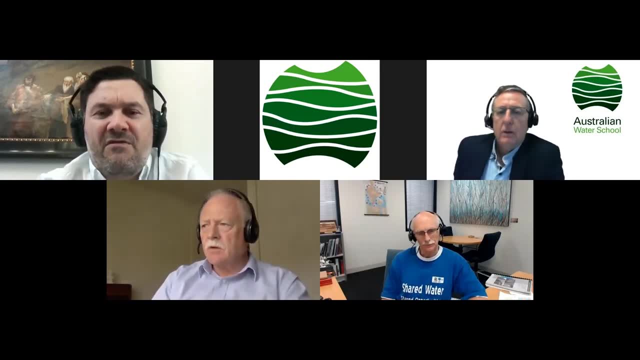 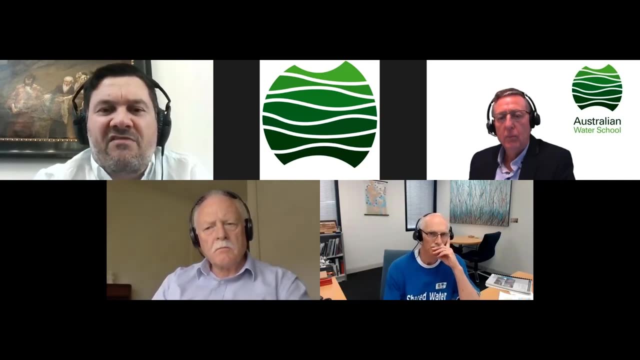 especially when it comes to human health and for irrigation and things like that. It could become a problem for many mass schemes as well if they become too pedantic in simply adhering to numbers. So yes, there are examples, And again these are with novel and emerging chemicals like PFAS. 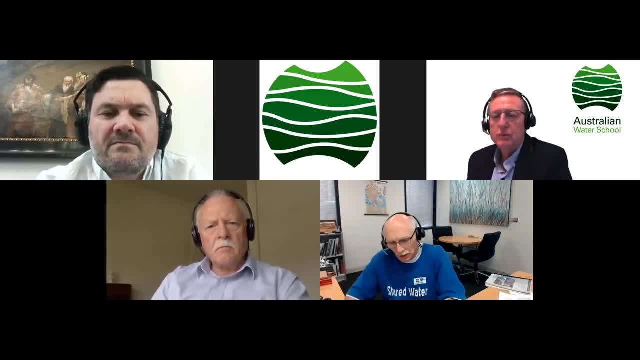 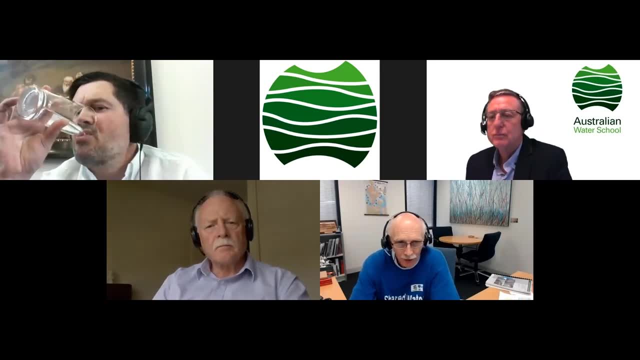 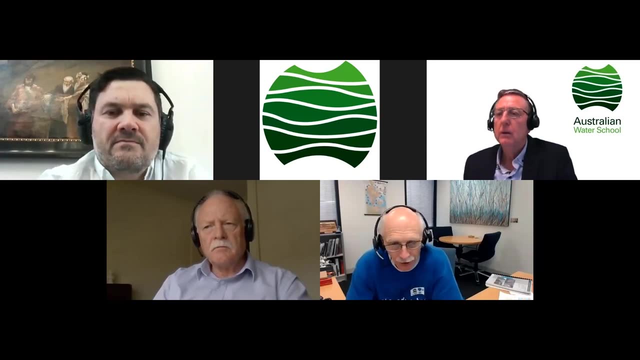 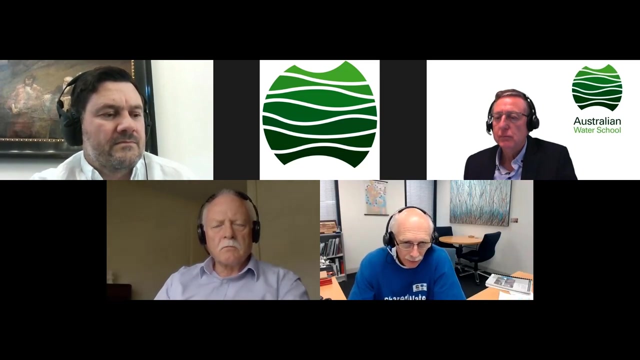 Thank you for the comment, Peter. Well, aquifers are not inert, and contaminants that enter aquifers can sometimes be removed. in the aquifer, For example, pathogens will often die off, and we can measure the rate of die-off of pathogens, And so you can work out how long it will take before that water would be. 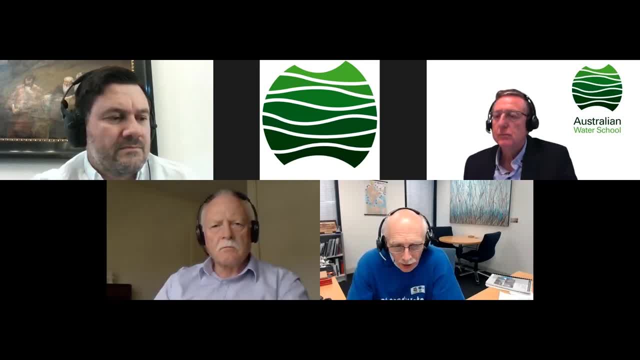 fit for whatever use you have in mind. And generally there will be a distance and attenuation zone set around those recharge wells or around a recharge basin that you would say: well, you shouldn't extract water within that zone because there's no guarantee that with the monitoring and the control that we've got on that stormwater. 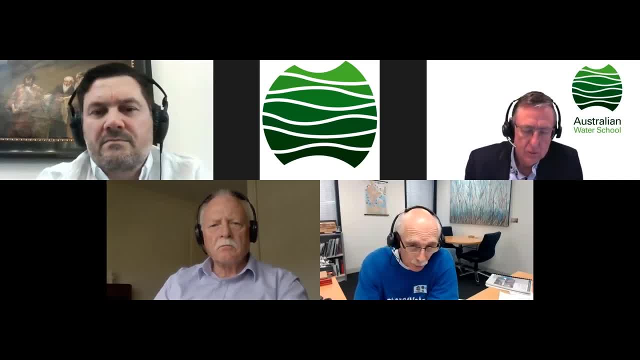 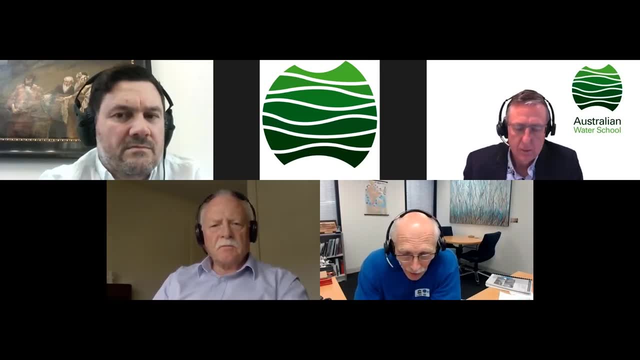 on that treated wastewater that the pathogens would be low the acceptable concentration for your intended use within that zone. But beyond that zone it should be, And so it's a natural attenuation process. There are other substances, some trace organics, that will sorb. 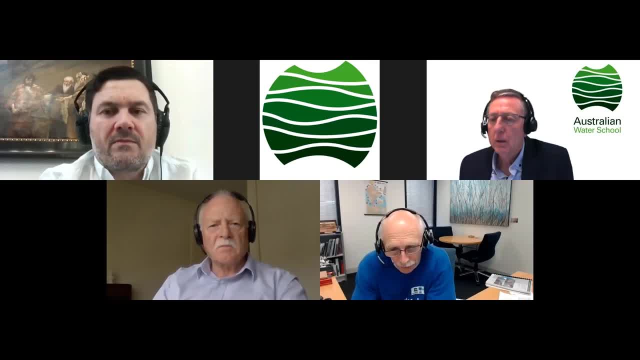 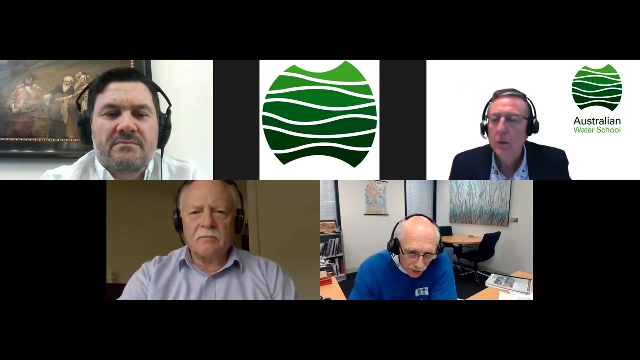 but we don't take into account the actual sorption of contaminants onto matrix as part of a sustainable removal process, because ultimately that sorption capacity could be consumed And then that trace organic might break through to recovery. well, So, understanding the aquifer system. 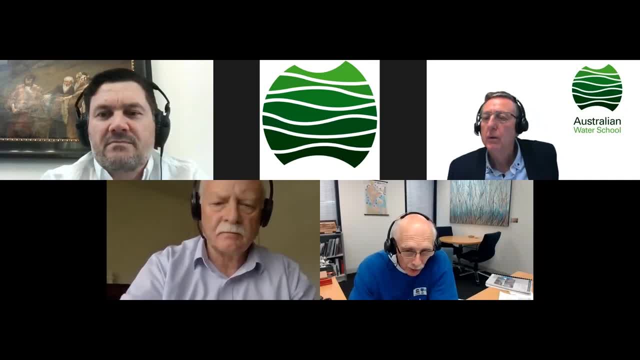 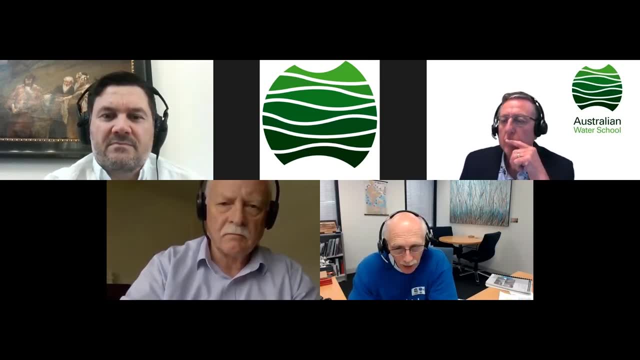 what the degradation is, whether the degradation process is a sustainable one, enables you to determine what level of treatment would be required or what level of controls would be required on the source water in order to meet the targets. So, thinking back to the diagram that Declan showed, 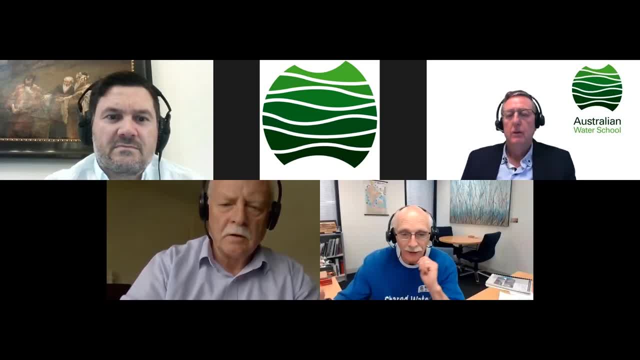 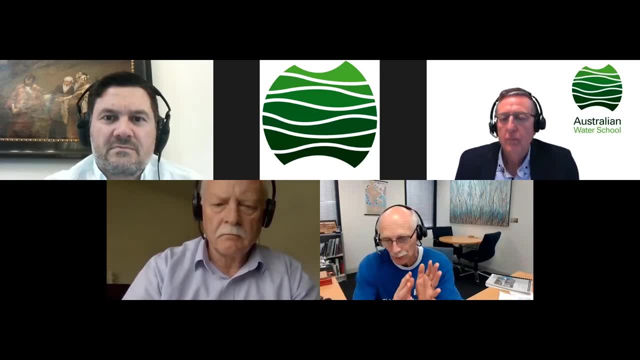 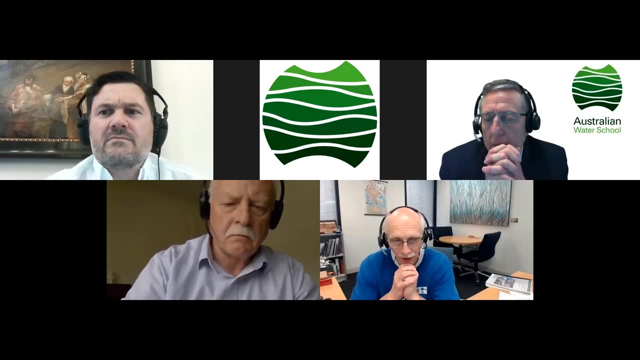 you can start with any source of water on the left hand side and get to any source any end use on the right, so long as you've got the risk management measures in place so that the water quality is improved to meet the requirements for its end use. 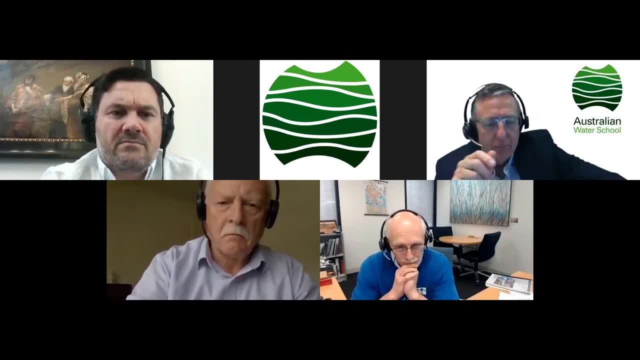 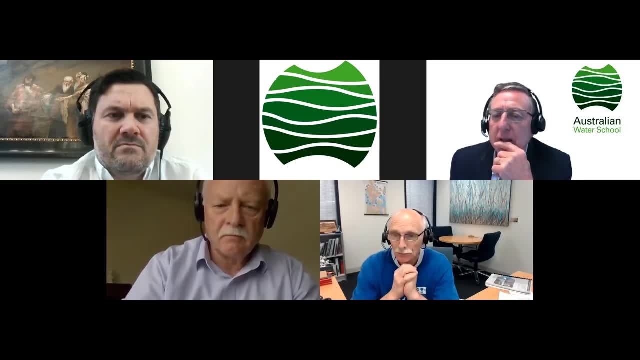 Thank you, Peter. We're nearing the completion. We've got two or three minutes before we hit our one hour mark, but there's probably one, two, three. There's probably three questions here. I'd really like to hit before we finish. 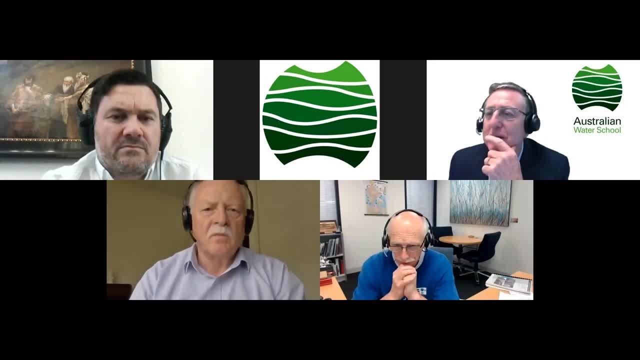 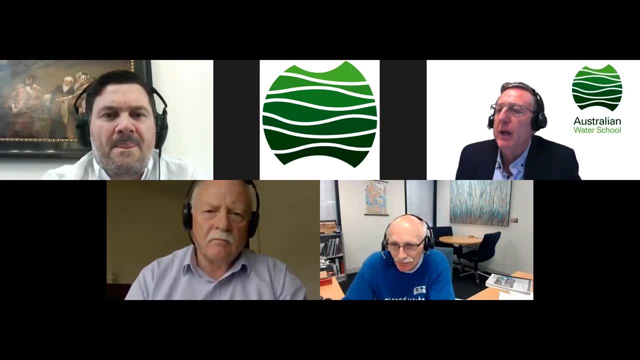 So there has to be brief answers to get this in two minutes, But the first one here from Nick Turner in the Water Corporation in WA, Western Australia. Does the panel have a view on how to allow for climate uncertainty in the planning and design of Mars schemes? 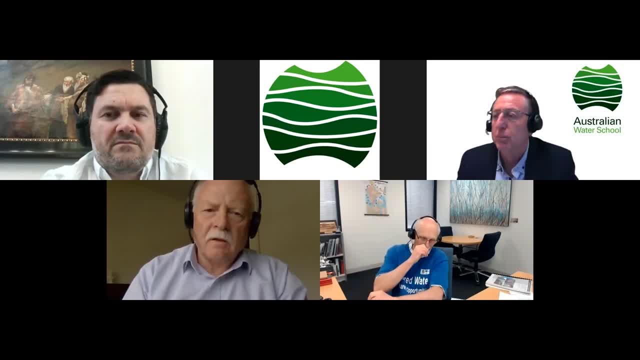 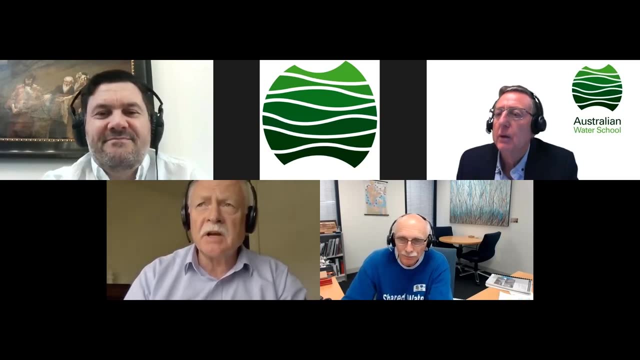 Big differences between dry and wet futures, as you can see. on that comment, So quick, probably one sentence answers: yeah, Yes, we do. It's absolutely critical to really get your source water modelling correct that takes into account the best available climate change scenarios. plus the changes that may be occurring through the catchment area, especially if you're looking at stormwater harvesting. Intensification of urbanised areas, for example, will also play a big role. We've recently completed some fairly detailed studies for one of our local councils in doing just that. 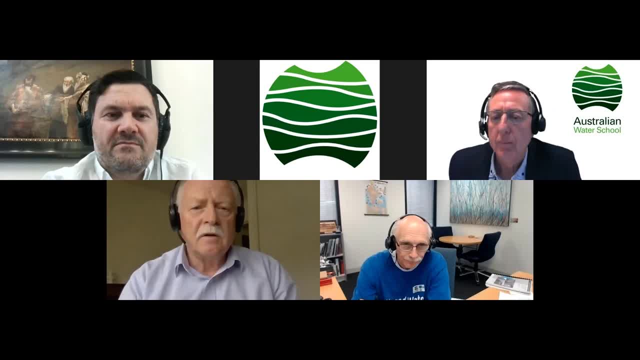 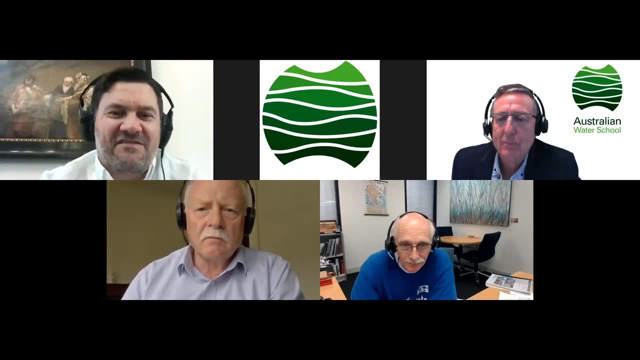 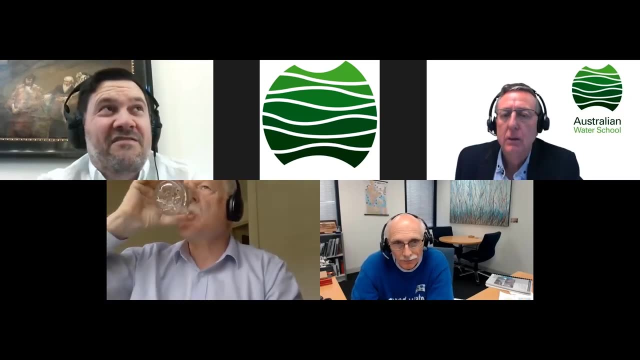 to make sure that we get it right. Yep, Any further comments? Declan: Yes, I've seen some great work that Dennis Gonzalez and Richard Clarke and others put out recently showing that stormwater harvesting is actually less- I guess it's more- resilient to climate change than thought previously. 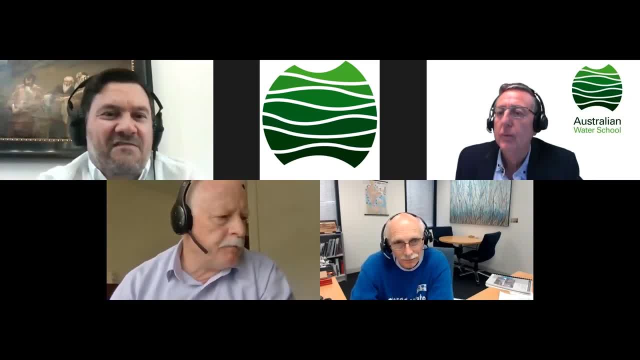 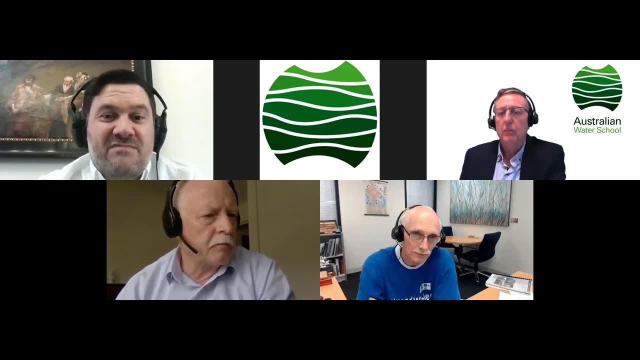 The increasing imperviousness, the sunny and urban catchments, the deaths, the decrease you see in rainfalls, showing that it is actually an effective method. And certainly here in Adelaide, where some of the modelling was done, shows that the declines aren't as bad as can be predicted. 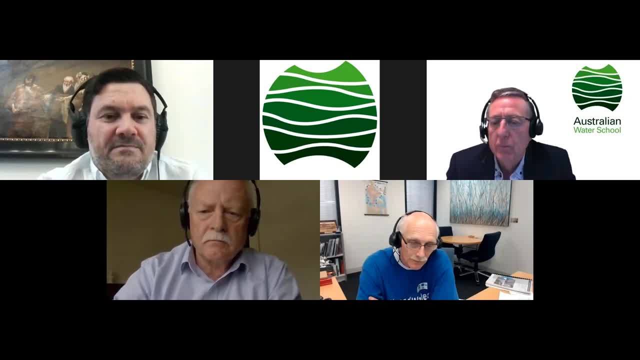 Certainly not as bad as in, for example, reservoirs. A comment, Peter: Yes, certainly climate change has to be taken into account as well as catchment changes, for whatever source of water you're using and whatever the demands are going to be on that water. 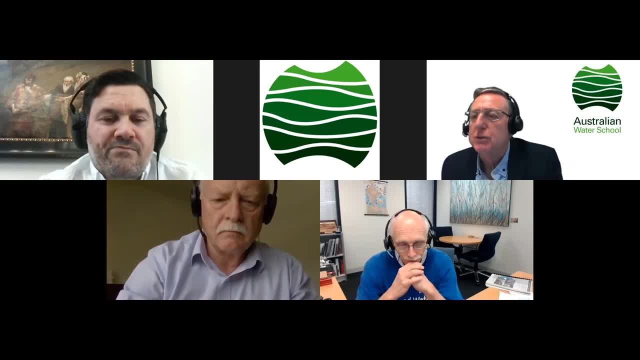 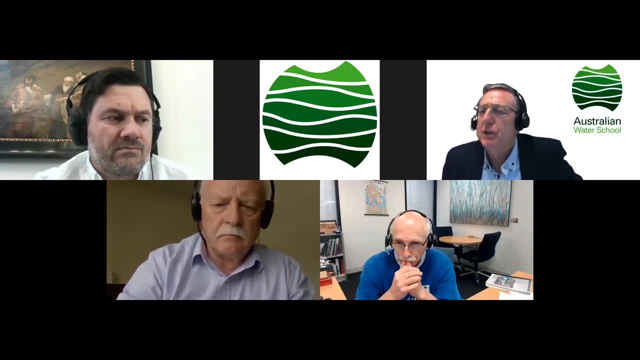 The next two comments. I think we'll take them as comments: Martin O'Rourke, New South Wales, and Simon Cruickshank, from the Northern Territory. Thanks for your comments. Martin says the water chemistry of the injecting water should match the water. 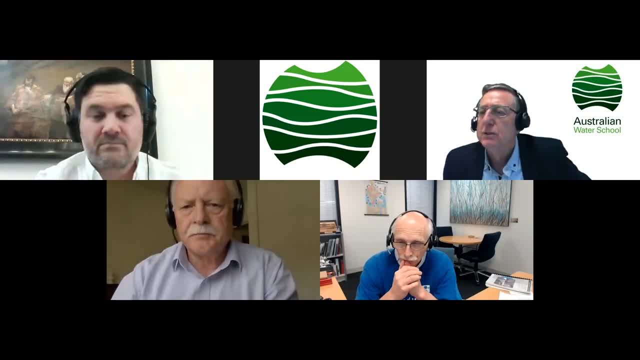 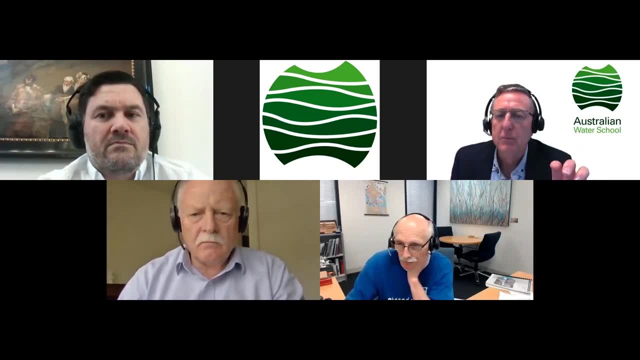 chemistry of the receiving waters, otherwise chemical clogging can occur. So all source water may need to be buffered to match the receiving water. I think we take that on as a comment. Happy with that, everyone Matching the source water with the receiving water. 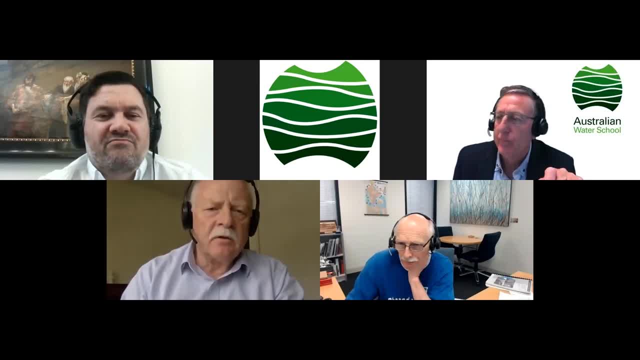 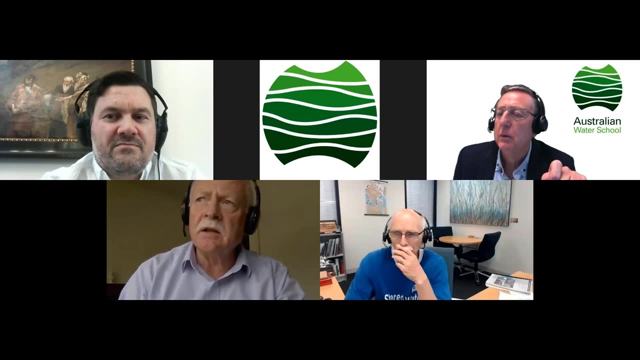 It doesn't need to be matched exactly. If you characterize your source water and characterize your receiving aquifer and your groundwater, then you can manage the systems. We routinely recharge fresh stormwater into high salinity ground water And there's a reasonable chemistry difference between our source and receiving waters in that regard. 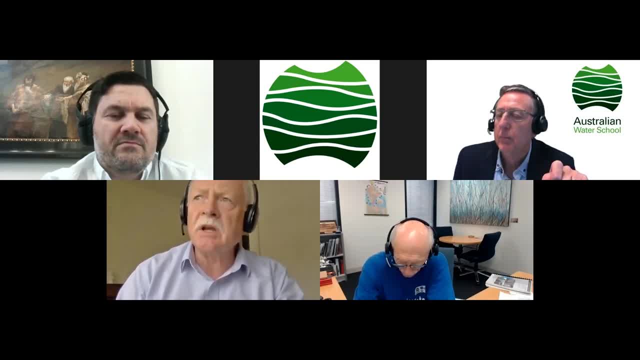 So it doesn't need to be balanced perfectly. But, yeah, just do your aquifer, Do your water characterization, your source and receiving water characterization to make sure you get it right and avoid potential issues with clogging. Comment: Declan Peter. 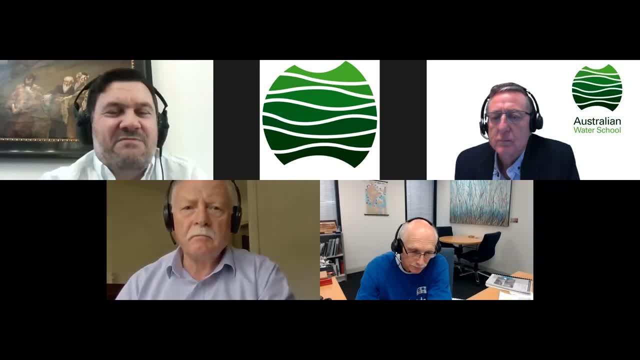 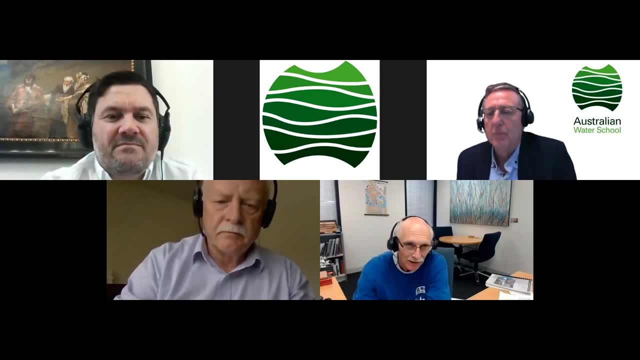 I agree, Russell. It doesn't need to be perfectly matched, But certainly there are elements of water chemistry that can increase in clogging, And those are probably the ones that you should focus on. Yep, sure? Last comment here from Simon. 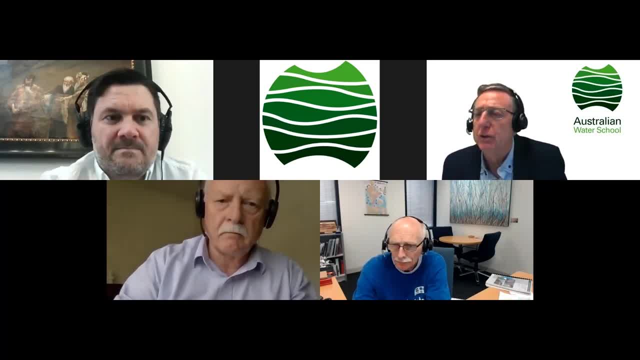 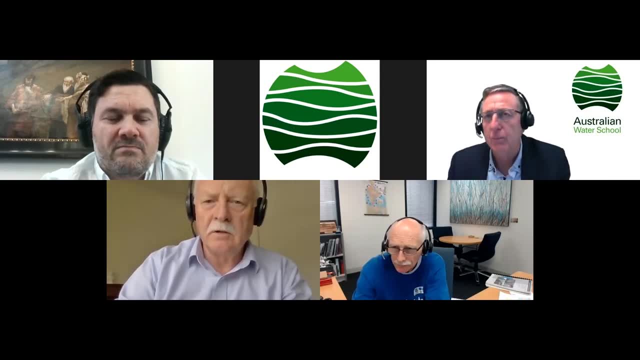 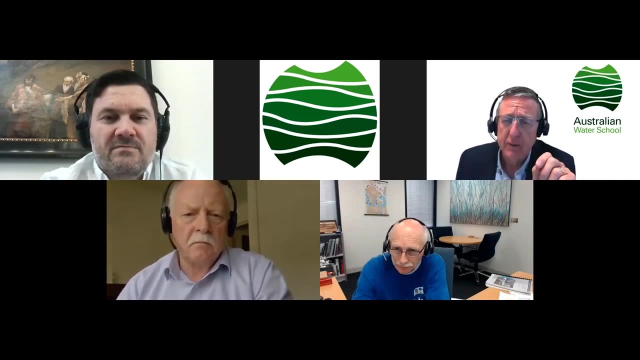 It would be useful to have links to well-written regulation policy documents for each jurisdiction. We don't have extensive experience in MA. We'll do that. We'll have on the web page for this webinar a resources section. In fact, if you go into the IceWarm Australia Water School website, 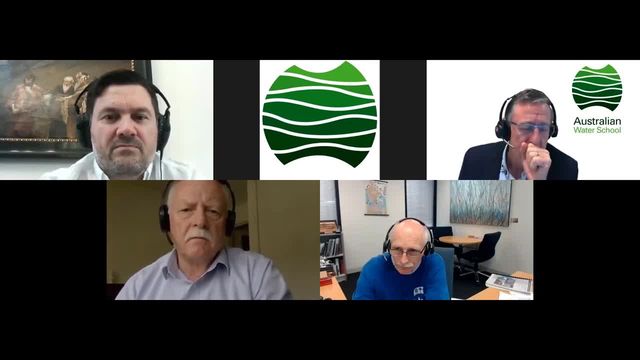 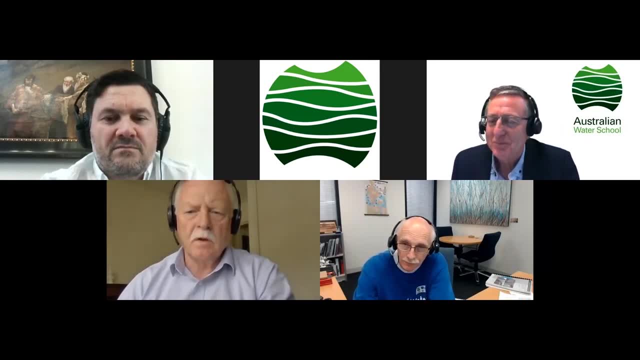 you'll see there's a resources section there. We'll put those documents up there. Excuse me, But look, I think we're going to call it a day for that. We've hit well over the one hour point, So we're just over the one hour point. 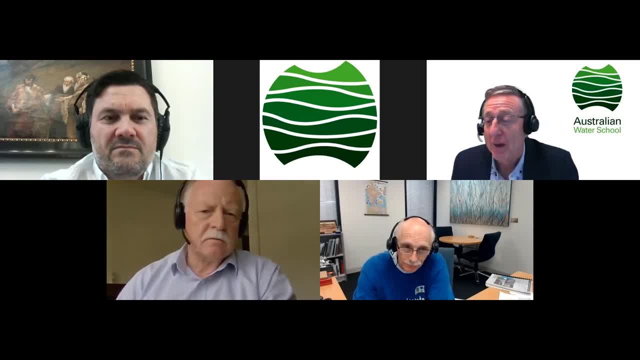 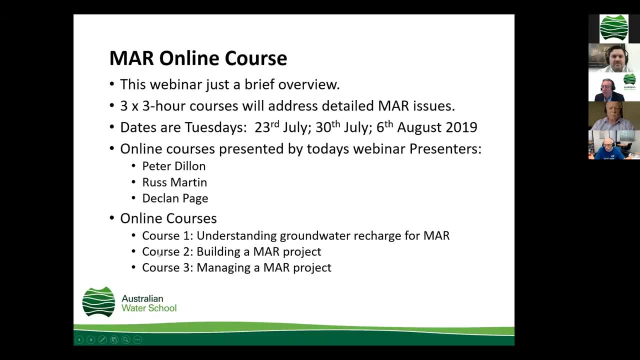 So we might leave it at that. Sorry, everybody. Thank you for your questions. Sorry, I've been able to get to them all, but I'm scrolling through them now. Samuel Waleed, Christo Guido. Thank you so much for taking the time to put these questions together. 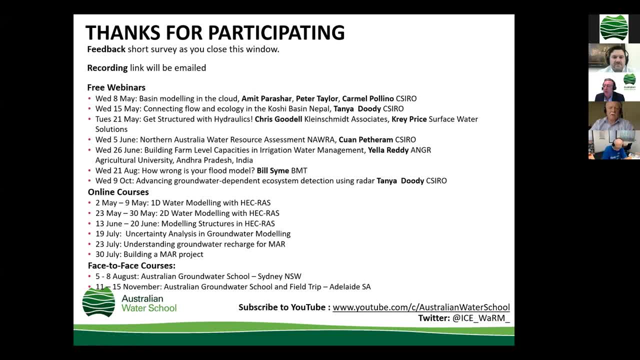 They'll still be on our file. We really appreciate your participation today. As you can see, there's a ton of webinars, courses and face-to-face courses coming up and online courses. There's a connection there to the YouTube resource. Subscribe to that by all means. 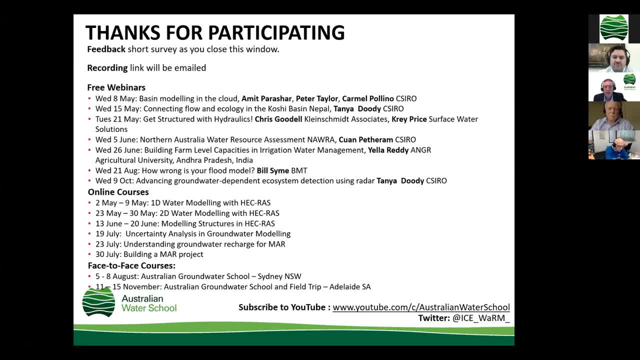 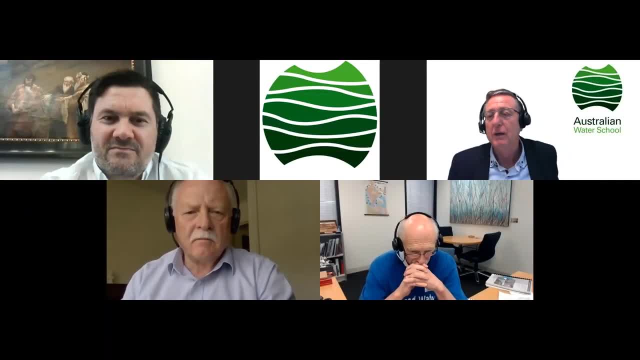 We'd love you to do that, And there's a Twitter address there as well. Any final comments from the three presenters about today's webinar? Where are we going with this MA training and capacity building? Kick off, Declan. I think you only really can scratch the surface in an hour. 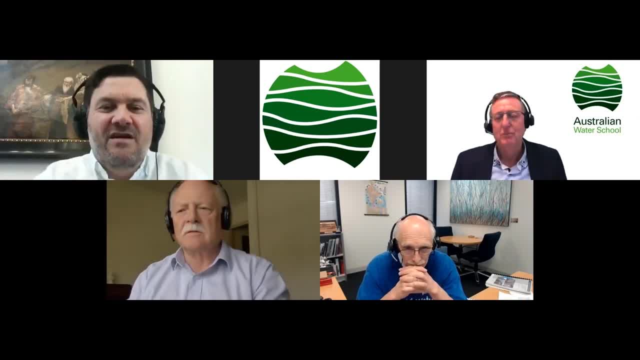 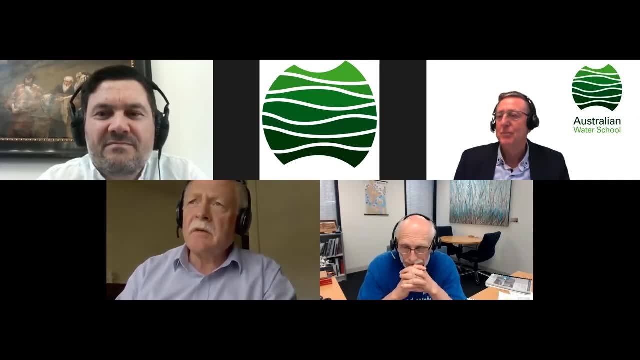 And, look, I'm happy to participate in some of the future courses and online schools that you have. Thank you, Thank you And Russ- Yeah, much the same as Declan, Having just come back from giving a test two and a half day workshop in South Africa. 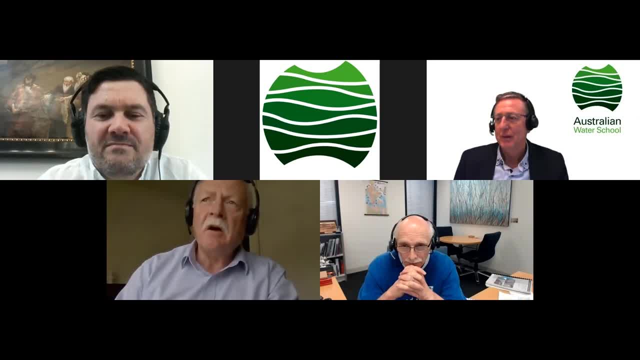 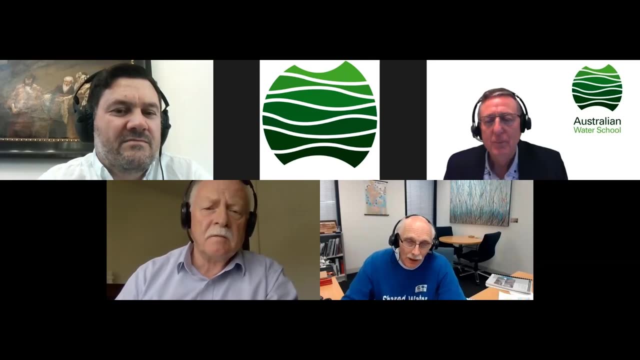 we really will only be scratching the surface, even in a three hour one, But all information- and this is a terrific forum for access to that information- assists in making sure that we can manage these schemes and implement these schemes going forward. Yep And Peter. 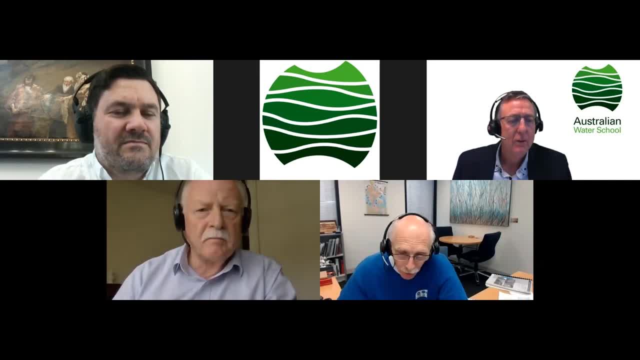 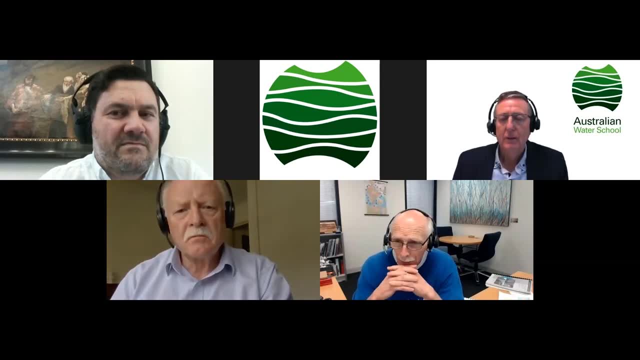 There's a lot that can be said, but there are some good resources available. The IHMAR website, Which I referred to earlier, will be on your notes. It contains those, In fact, Simon Cruickshank's question about regulation and policy documents. 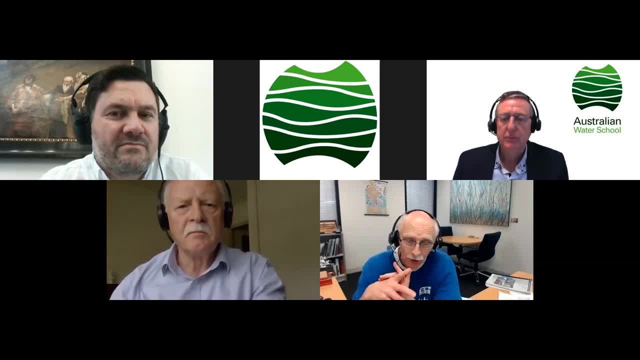 There's a collation of them already on the IHMAR website So you can look there. So I think the questions we'll be answering in the future they're going to be different from the questions we're answering today Because of things like climate change. 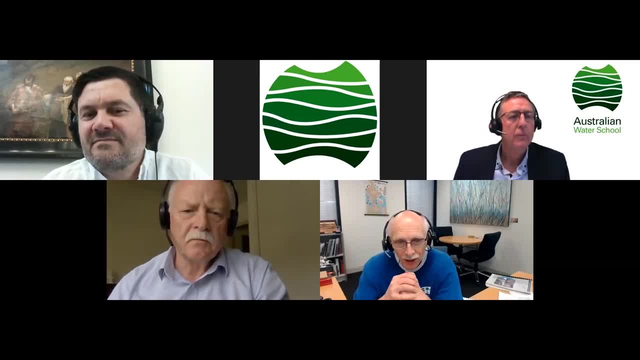 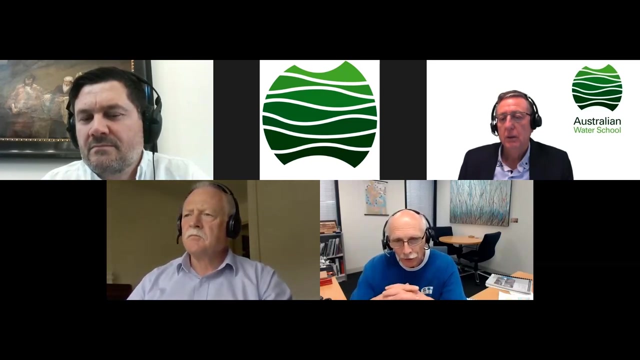 because of changing catchments in urban areas and densification of cities and so on. But I guess if we build capacity then we could adapt. If we understand the principles behind things, as Russell and Declan have been saying, then we can make advances. 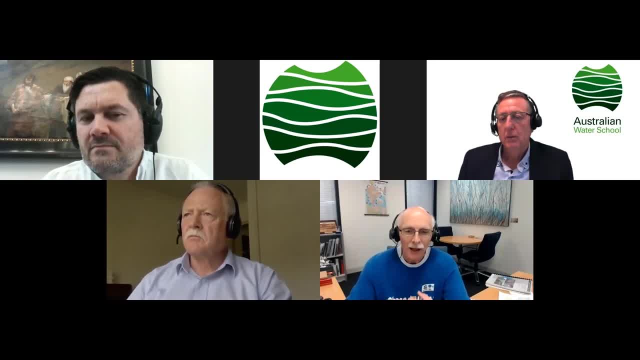 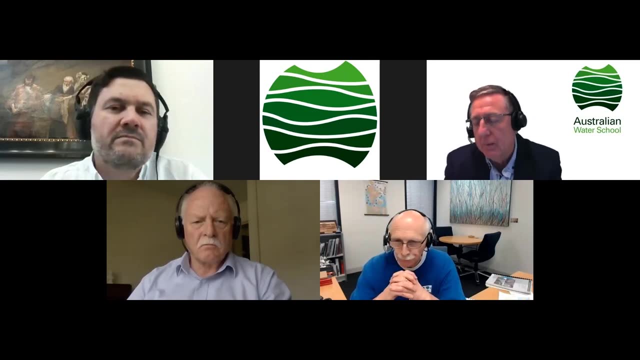 It's not just a matter of copying what they do in Australia. It's adapting to in your own circumstances to do what you need to do to best meet your needs. That's fantastic. We absolutely appreciate the extensive experience and knowledge coming to bear here today for one hour.